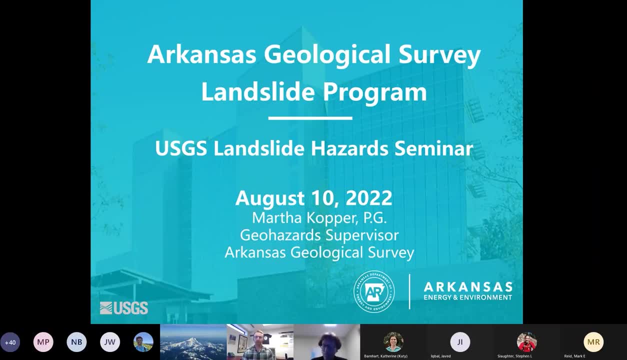 where we hear from our state surveys. These talks provide an overview of state landslide experience, focus areas, product types and introduce some of the most pressing landslide related problems that our states face. If you'd like to have your state landslide work spotlighted as part of this meeting, please do so. 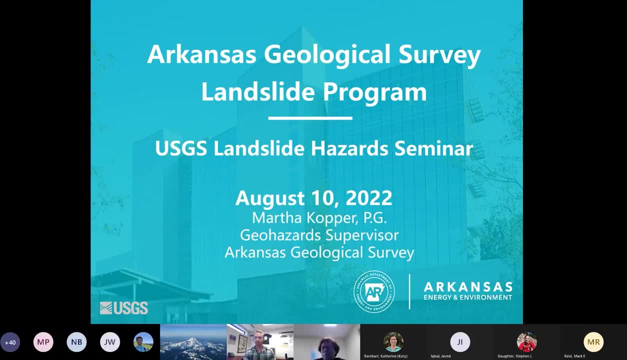 Today we're joined by Martha Kopper. She is a registered professional geologist in Missouri and Arkansas. She received her BS in geology from Southeast Missouri State University, her MS in geology from Wichita State University and is currently working towards an MS in. 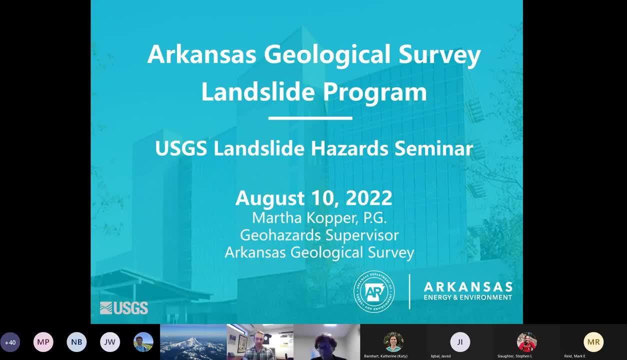 geological engineering at the Missouri University of Sciences and Technology. She serves with the National Geological Survey as a geology supervisor, focusing on landslide and earthquake geohazard research. At the present time she is working with local regional county state. 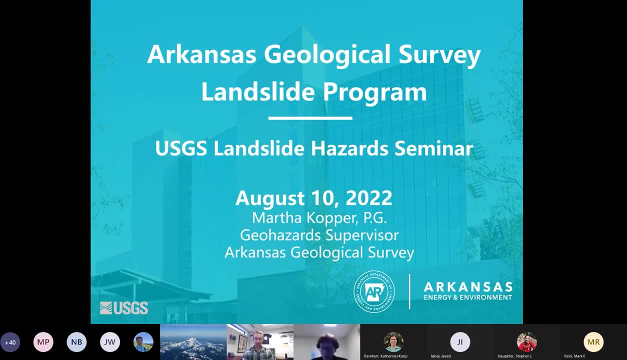 and federal organizations and landowners to develop a landslide geodebate database across Arkansas, with assistance through two grants. Findings from this work will be summarized in an all-hazard mitigation plans for areas covered by the grants and as part of those grants. 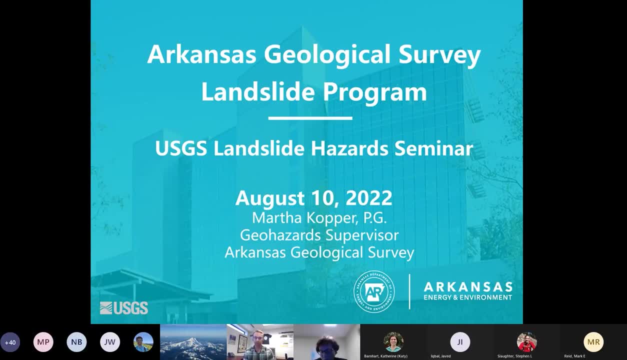 she's working with MS and PhD graduate students whose interests lie with landslides, landslides and landslides. She's also the chairperson for Arkansas's Governor's Earthquake Advisory Council and works closely with the Arkansas Division of Emergency Management. 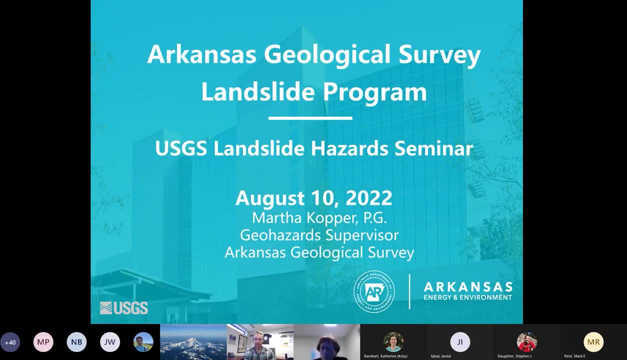 and the Central United States Earthquake Consortium. She also manages a multi-state induced landslide seismicity earthquake grant and has served on the Association of Engineering Environmental Geologists National Board and is a member of the Seismological Society of America and American Society of Engineers. A lot of accomplishments to list there, Martha, Thank. 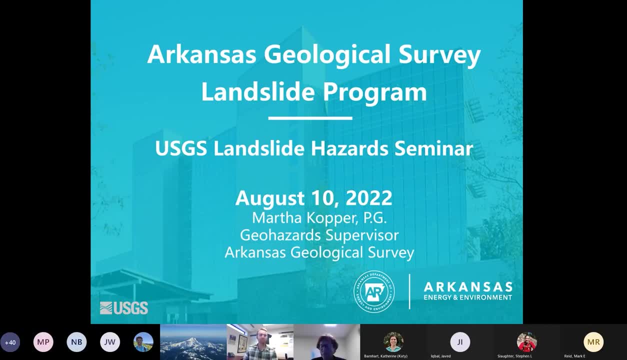 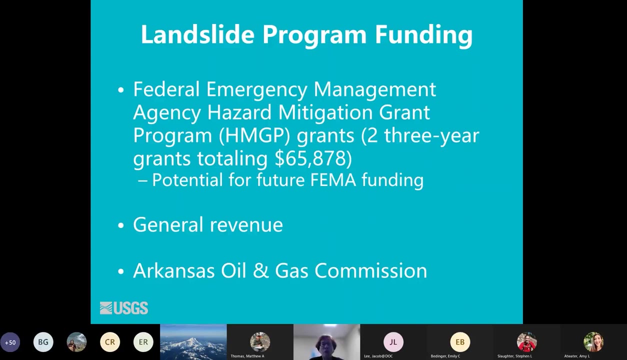 you very much for joining us today. I'll go ahead and get started. Thanks very much. So thanks for the opportunity to present our program. So I wanted to start off with what our program consists of. We have a federal emergency grant that we received. It's 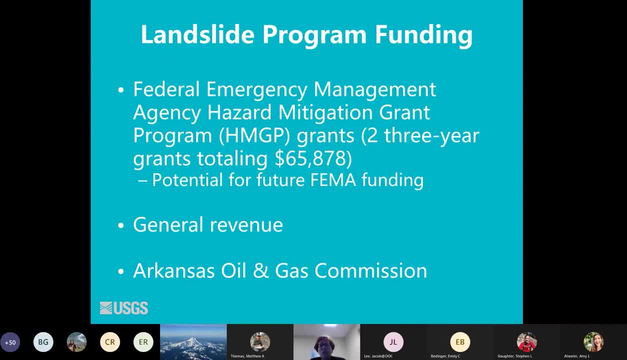 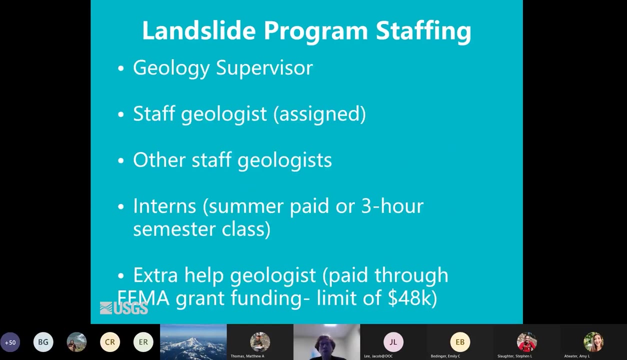 a two- three-year grant totaling about $65,000 with a potential for future FEMA funding. We're also funded with general revenue And some funding from the Oil and Gas Commission. Our program staffing consists of myself, a staff geologist who's assigned, some other support staff, some interns and an extra. 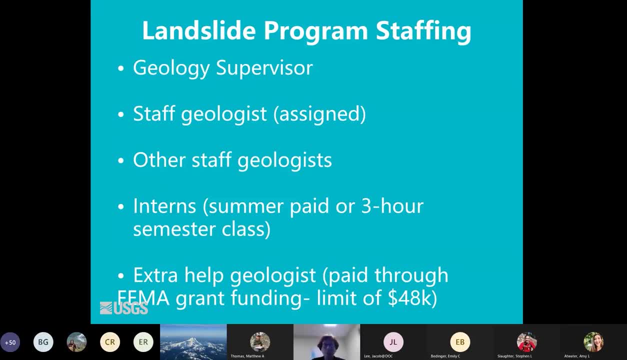 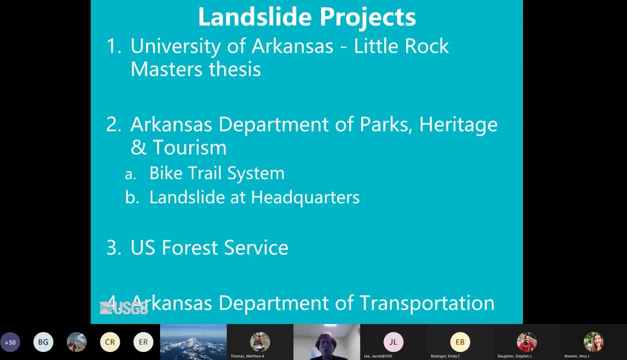 health geologist paid through the FEMA grant. So I'm going to list out several projects that we're currently working on. Some of these we've just recently completed, So we'll just these relatively quick. So first off we're: I'm working with a master student with the University 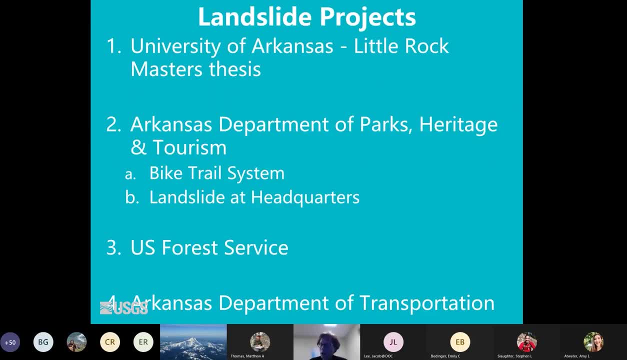 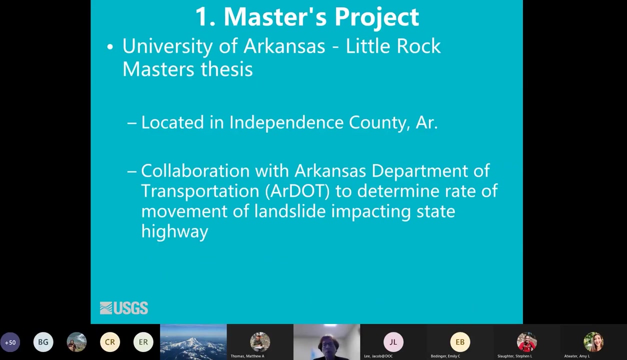 of Arkansas, at Little Rock. This master's project was developed by developed in association with the Arkansas Department of Transportation Engineer, And part of it was funded through the RDOT research money that they had set aside, And so it's located in Independence County, which is kind of in the northeast part of the state, And so we're working with a. 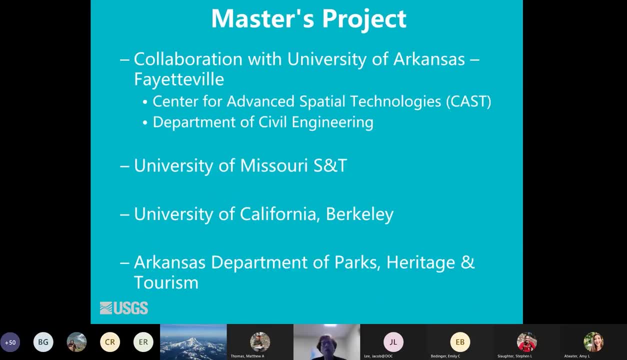 of the state and we're working this. so this project, we're working with the university of arkansas at fayetteville in their cast, our center for advanced spatial studies, technologies and also department of engineering, and we're also working with university of missouri science and technology. 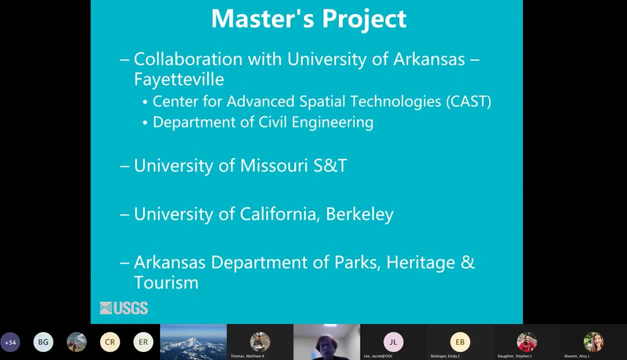 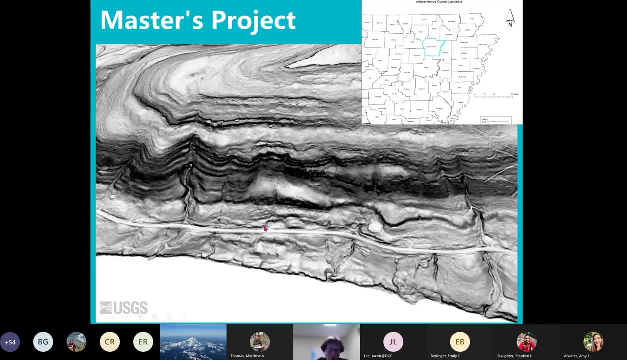 university of california, berkeley, and the arkansas department of parks, heritage and tourism, and here is the project site. so i have a pink cursor here. so, um, the highway department has put in um a somewhat of a mitigation, retaining uh wall here, and i'll show you that here in just a second. 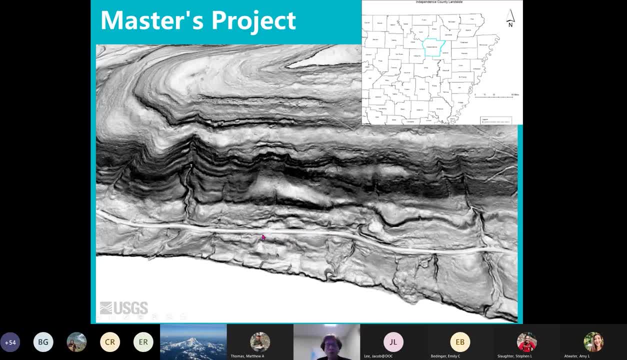 so this is about i don't know half a mile long. they put this um mitigation in because the the hillside was failing and the master uh project is essentially flying a drone with centimeter resolution lidar over this area that i'm kind of highlighting in here. as you can see, this is an old landslide here as well as actually. 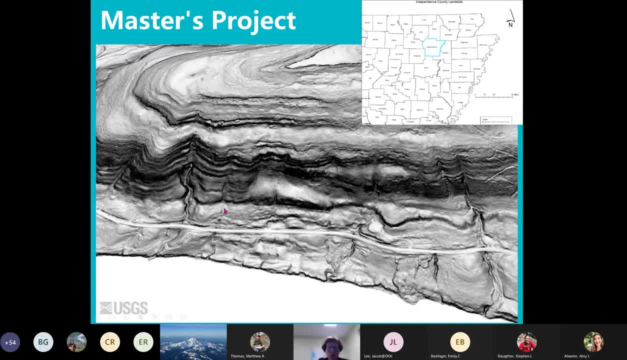 pretty much this whole slope. i'm going to explain the geology to you as well. so approximately here is where this elevation, here is where the fayetteville shale contact is, and above there is what's called the pit. uh, that um, and so let's advance this. um. i wanted 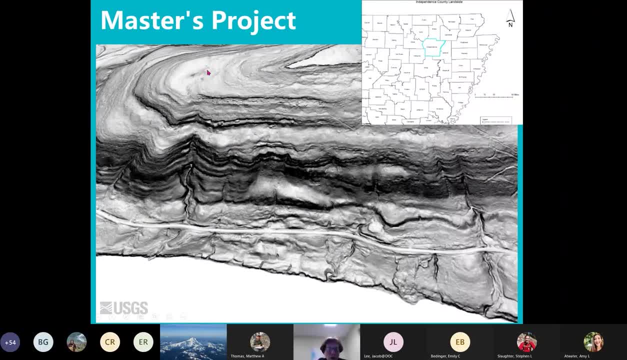 to point this point out right here. this is part of the pitkin, it is um, it's karst, this is a, this is a sinkhole actually here and then back over here is a cave, and the reason we're working with the department of parks is because this cave has some endangered species in it. so this is part of. 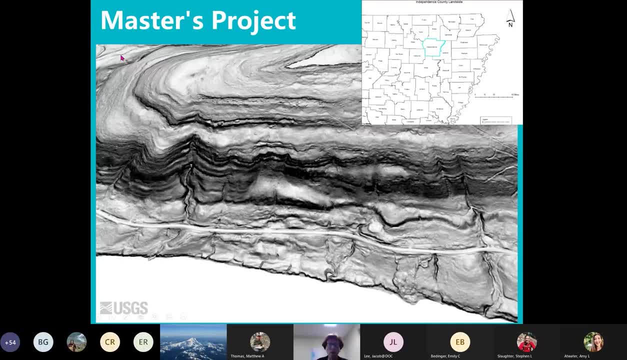 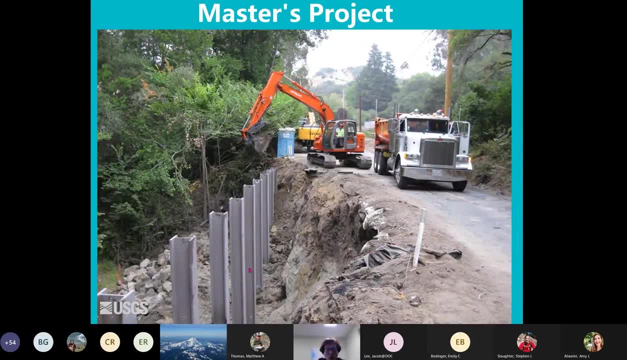 their um uh area that's susceptible to. so this is the mitigation, similar to what the highway department is putting in. they put in rails and then sheet um sheet metal in here to the batesville formation and it essentially prevents um or holds back some of the slide um. so this is the the pitkin. 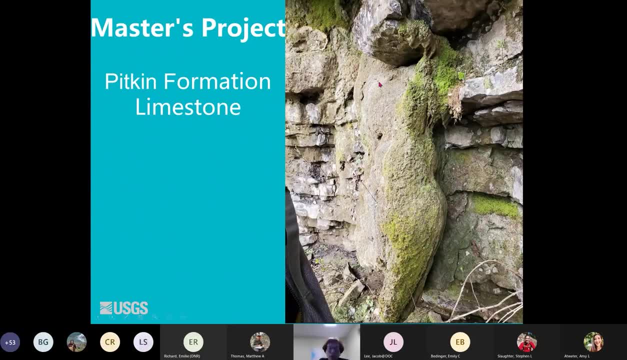 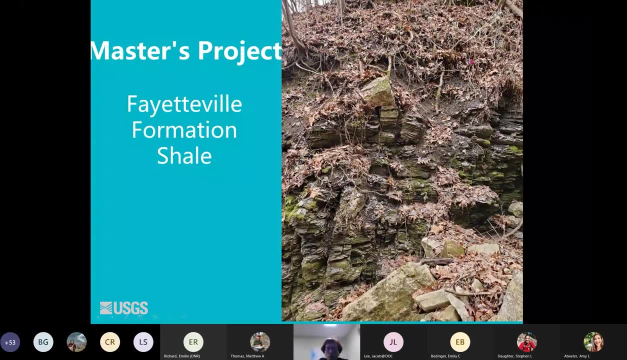 formation which overlies the, the fayetteville. so the pitkin is a limestone and this is the formation that the cave system is in. this is the fayetteville formation, so you can see a lot of ting um. so what we believe, one of the triggers for this landslide um is um the cave system. 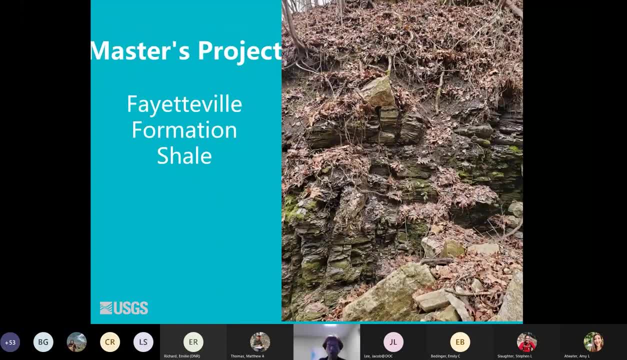 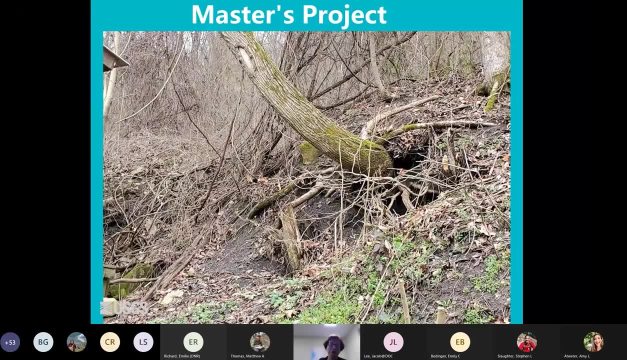 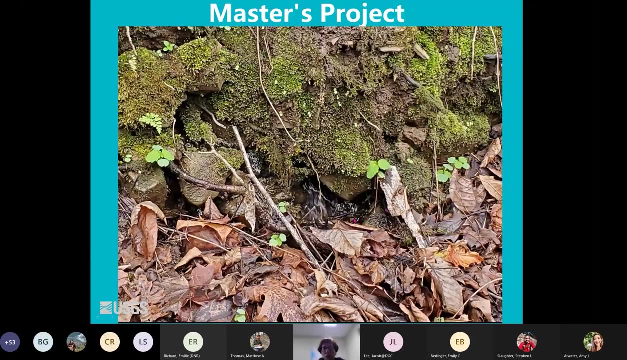 um percolating groundwater through these fractures and joints in the fayetteville. fayetteville is a shale and here's some of the uh tilting trees. um we another thing i found was um a right after a rain. we went up there and looked to see that the roots were providing an avenue for. 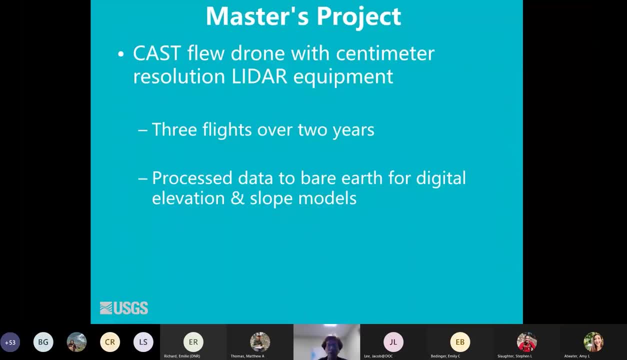 the groundwater to, to percolate through that that landslide. so, as i mentioned, the um, the cast flew a drone with centimeter resolution to deter over um three flights over two years, process it down to bare earth, got the digital elevation and slope models and what the master student and 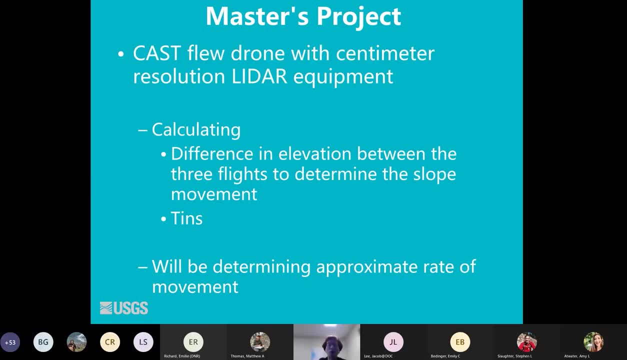 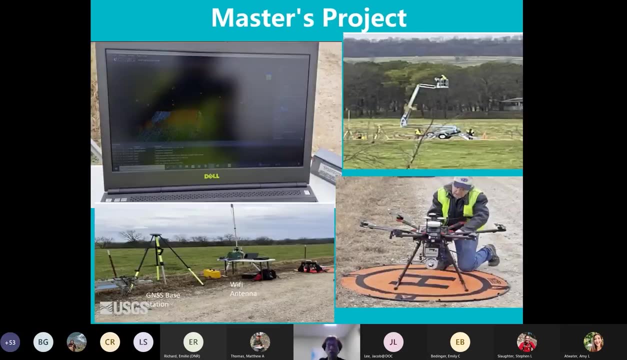 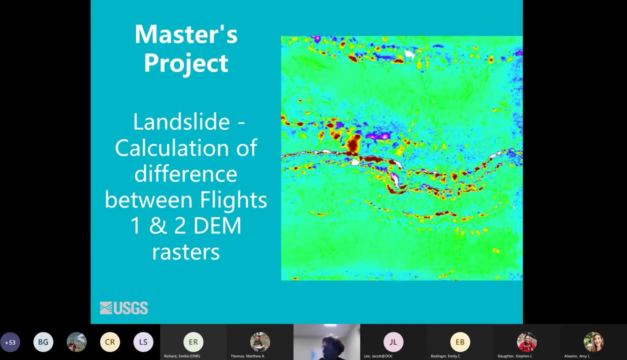 working with him to determine the elevation difference between the three flights, to determine the slope movement. essentially, the highway department wants to determine the rate of movement. so here's their setup, pretty, uh, pretty incredible here and um, they here is, um, this is the first uh iteration of the calculations, um, so there's some. we had some problems with some of the. 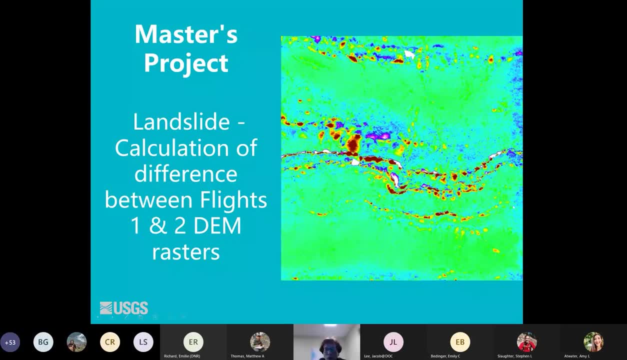 um, the otheridan, and then also some of the other visions and slides that i put together, um, but, as i said, we- there are also some um and the the other in the other repairs were also very important, but we all know that, uh, that, uh, as you can, if you were to get a small. 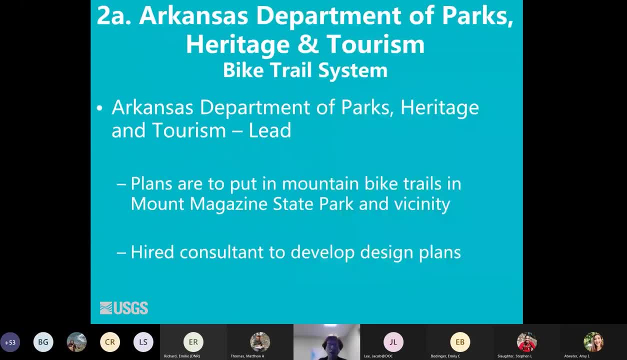 acre of land, for example. you know how many acres you can get. um, they're getting like about 20, so it's a. it's a pretty key problem if you could divide that up, you know, by that number of blocks. right, and this is all there on the map. so if you were to get a, uh, the 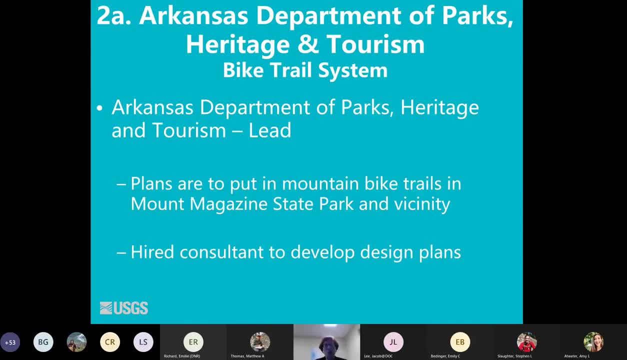 uh, the, the level of, uh, the level of reuse was 15.5, so you could get at least 15. so we They have this mission to establish a really nice bike trail system throughout the state And they had a consultant who contacted us and they wanted us to help them map out all the landslides. 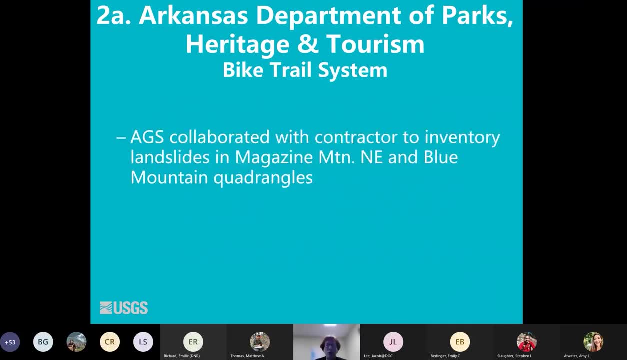 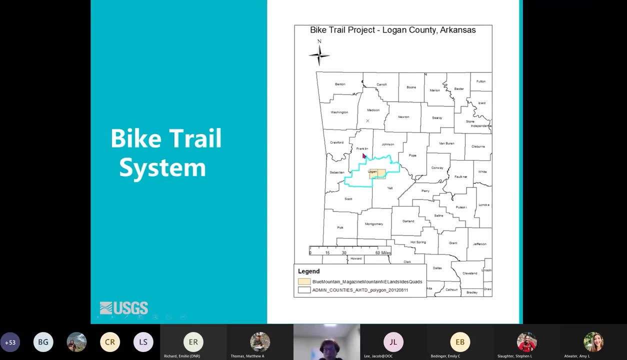 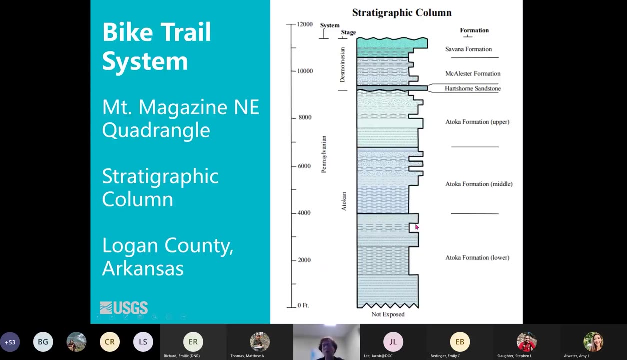 And this is in a park called Mount Magazine, And so it is located in western Arkansas. Here it is in Logan County, And I want to explain the stratigraphy of the area. So we'll see a common theme throughout here. In the areas that we're mapping, it's mainly shales. 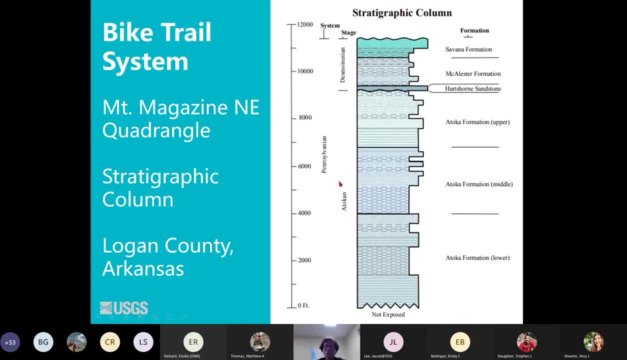 So this particular section is within the state park but it does not extend farther away from the area. But at any rate we have the McAllister. There's some coal- small coal- seams in the heart surrounding McAllister, But below there we have the Atoka. 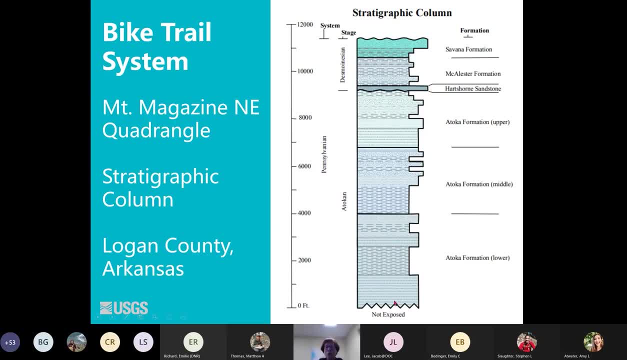 And then north of the state park we have the Bloyds. Anywhere where we see blue, it's going to be shale. The Atoka is a series of three benches of sandstone separated by shales, And it is very susceptible to failure. 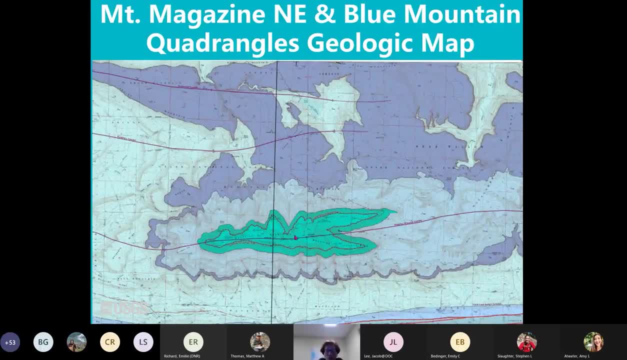 So, as you can see, the state park is this greenish area, So this is the somewhat substantial sandstone on the top, And then the Atoka is this bluish gray around here, And then the Bloyd is this purple color in here. 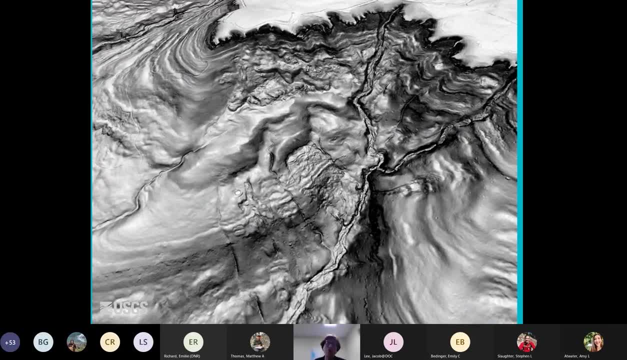 So here is some LIDAR from the top, So this would be the McAllister, And below here is the Atoka, So you can see some flow, a lot of mass movement on these slopes. This is one meter LIDAR. 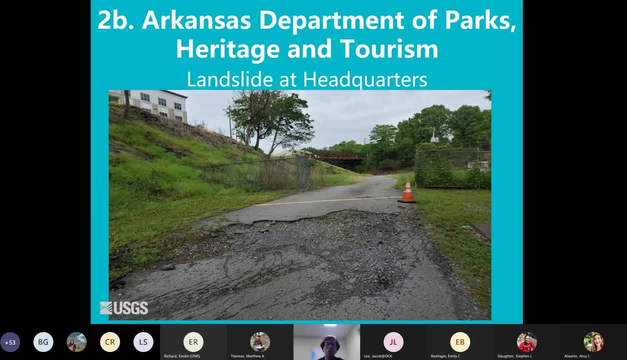 The second Department of Parks, Heritage and Tourism project was a landslide at their headquarters. So off to the left here you can see their main building. It's right on the edge of this bluff. This is this. Here, Where my cursor is, is where the SCARP for this landslide is evident. 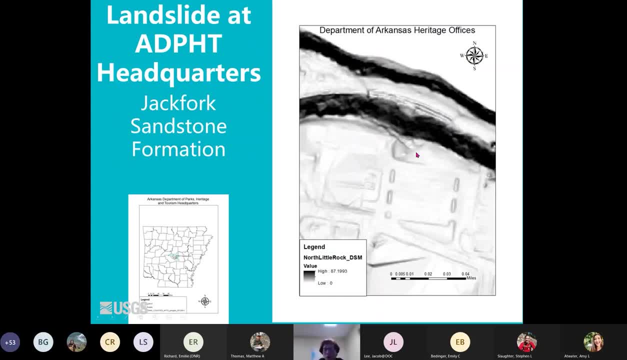 So I pulled up the one meter LIDAR and you kind of see where this landslide is. This is on the Jack Fork sandstone formation. This particular formation is dipping very steeply, So this is a dip slope scenario. This particular formation is dipping very steeply. 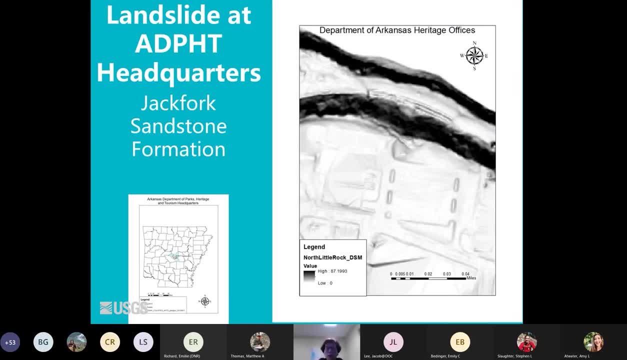 So this is a dip slope scenario. So this is a dip slope scenario. So this is a dip slope scenario. It's dipping at like 45 degrees And this is right along the Arkansas river, Pretty near downtown Arkansas, So it's in the center part of the state. 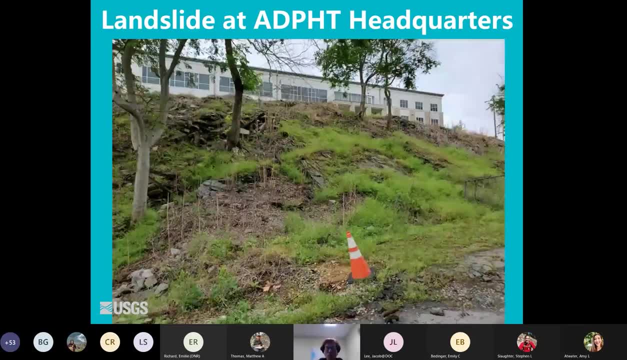 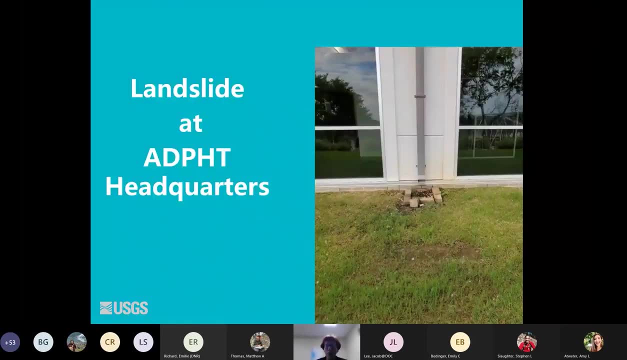 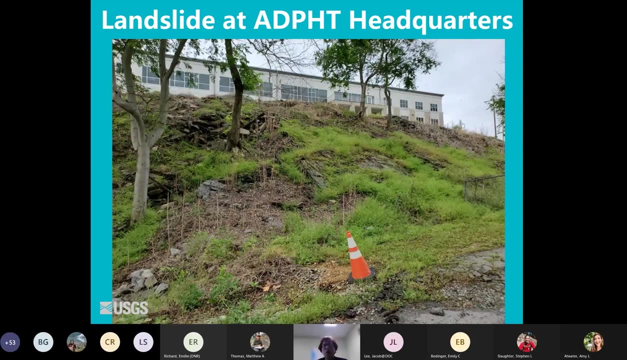 Here are some trees that are leaning here. you can kind of see the dip slope here. I was asked by the folks there at the agency to come and take evaluation, to come and take evaluation, evaluation, take a look at it, and I wrote up a paper for them to provide to their engineer. 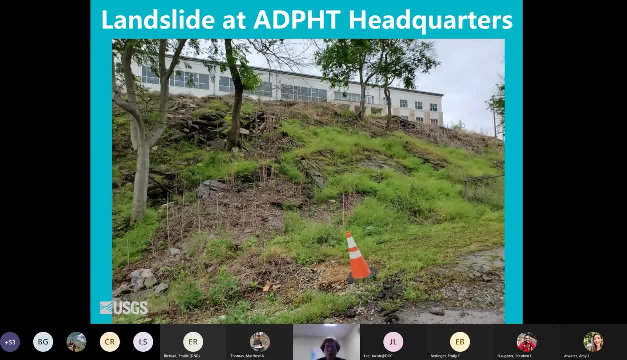 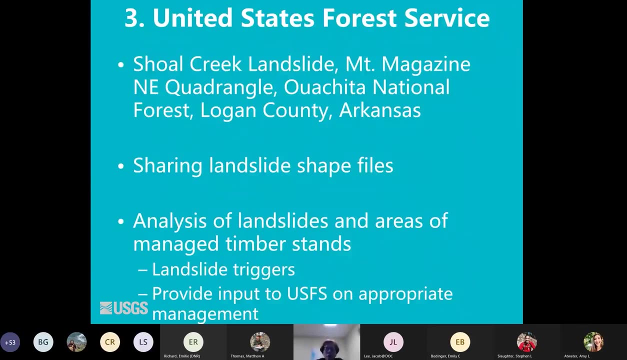 their contracted Engineers and I noticed that they had drainage or downspouts all along the the back side of this building. so, uh, I made that in my recommendation. um, so a third project is working with the US Forest Service. one particular landslide we looked at was Shoal Creek. it's just. 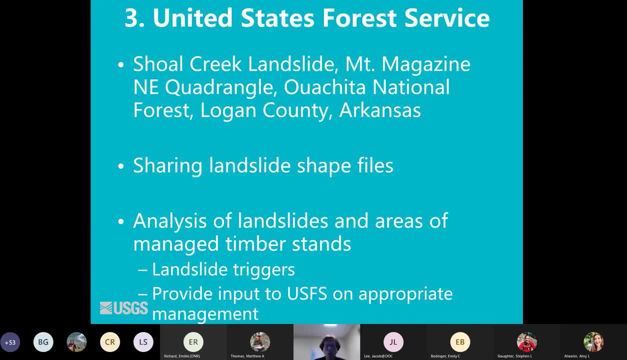 north of Mount Magazine, where we just looked at a while ago. we're sharing shape files with the Forest Service and they have shared with us um shape files are their managed timber strand stands, and so we're going to be evaluating that as well at some point. so here's the Shoal Creek landslide. 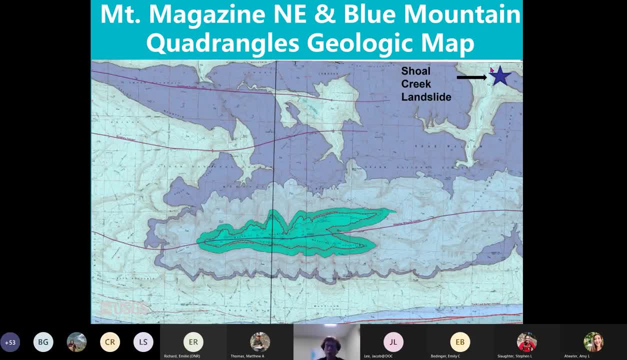 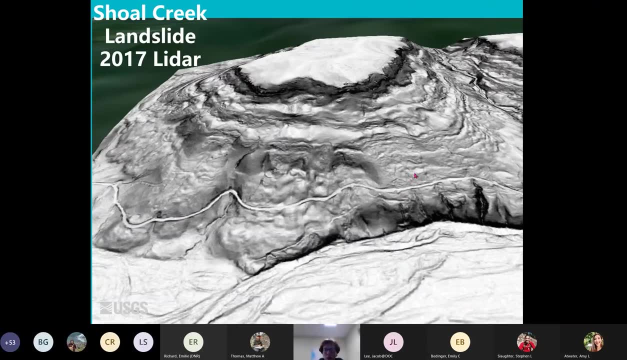 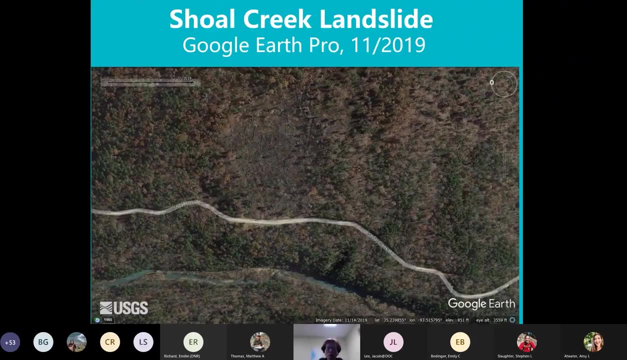 up here. it's within the Atoka formation, so this is a Forest Service land here. this landslide we're talking about is right here, and so that's 2017 LIDAR. this is a 2019 Google Earth, so you can kind of see this older footprint. this is 2020 and it was kind of funny the landslide left a little. 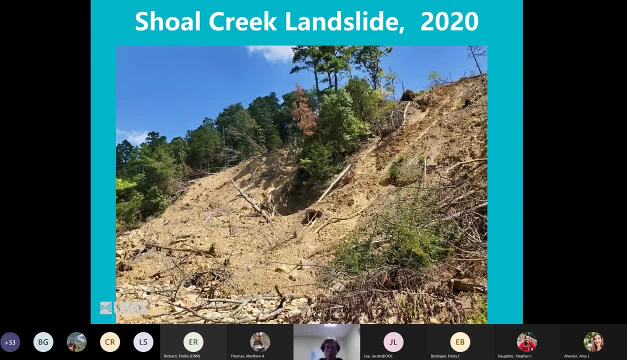 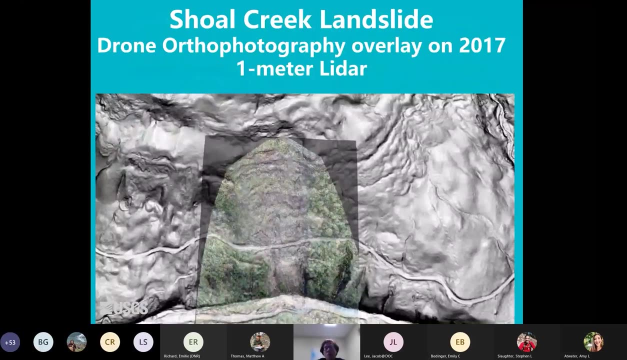 island here in the center, um, and it completely destroyed the road, the US Forest Service road, and, in addition to which it um backed up the lake and formed a little lake there, um. so here we, we have drone pilots, um licensed drone pilots, and we went out and they took some. 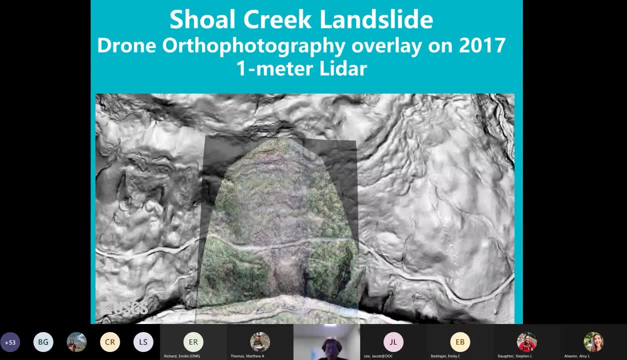 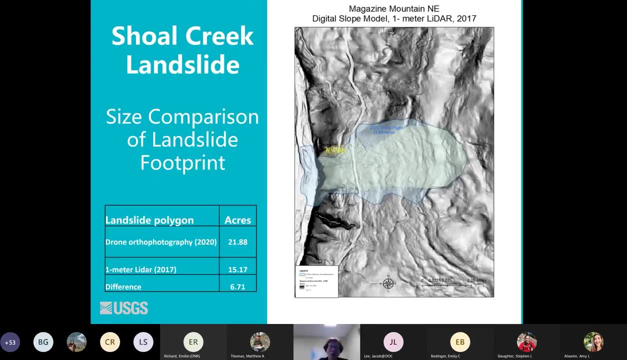 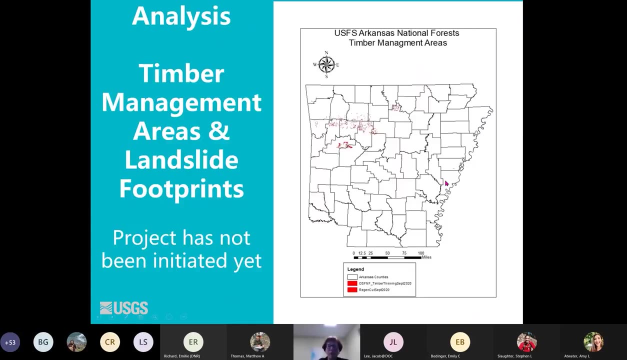 photographs and we mosaicked it and um overlaid it on top of the LIDAR to see the size change in the landslide and it's about almost a seven acre increase in size of the footprint of the landslide. as I mentioned, we're going to be doing an analysis with the US Forest Service shape. 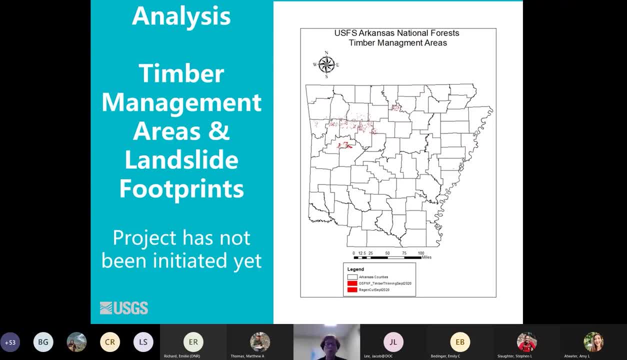 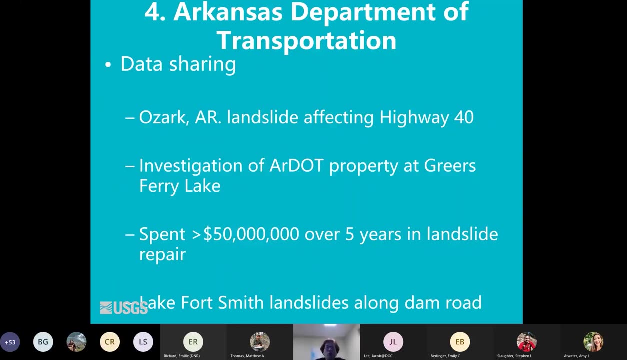 files with regards to where they've cut down the trees, where they've done controlled burns to see if there's any sort of a relationship between the landslides and their management. the next project we're working on is with Arkansas Department of Transportation. we looked at a landslide out near Ozark, Arkansas, that it's kind of interesting that the highway department 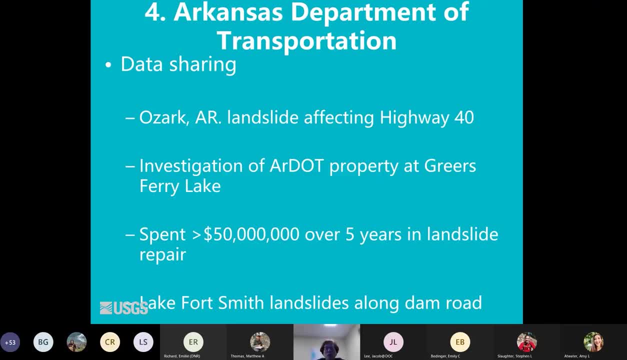 has spent over 50 million dollars over a five-year period in landslide repair. they've been doing an inventory themselves on not only the landslides they've repaired but also future work that they have. that in speaking with the, the engineer that I'm working with, there he goes. this is my lifelong mission. 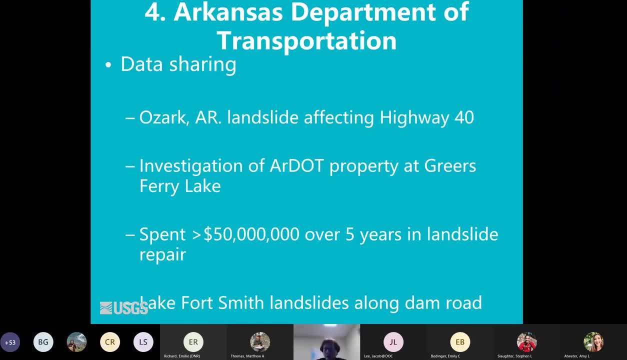 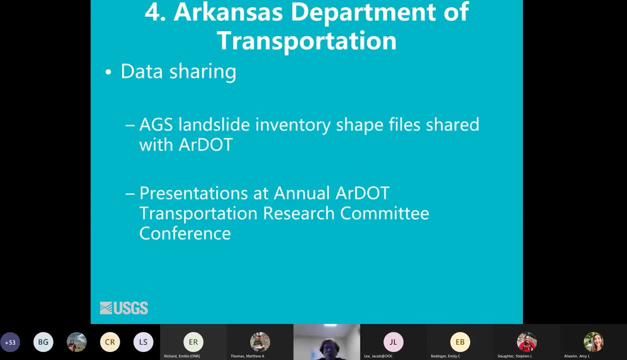 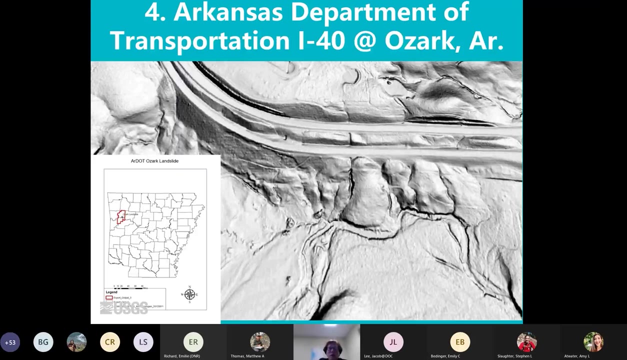 is to rid the state of landslides along the highway corridor. so we're, of course we're sharing the inventory shape files with them and we've also give presentations at their research conference. so here is the Ozark landslide right here. it's kind of in the western part of the state, and what happened here is when. 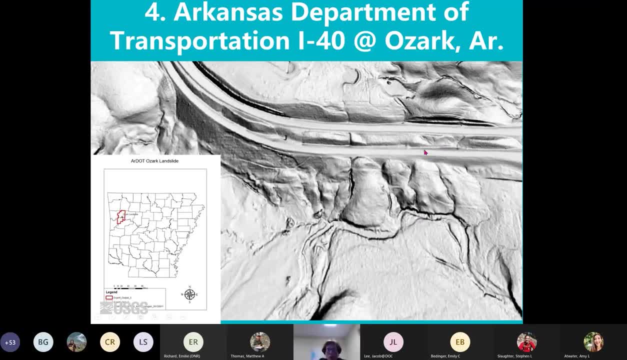 they first designed and built 40 through here. it was a little hilly, so what they did was a cut and fill, and so the fill now acts like a bathtub, and of course this is on susceptible shales, and so what's happening is the shales are filling up with water and then the pore pressure changes. 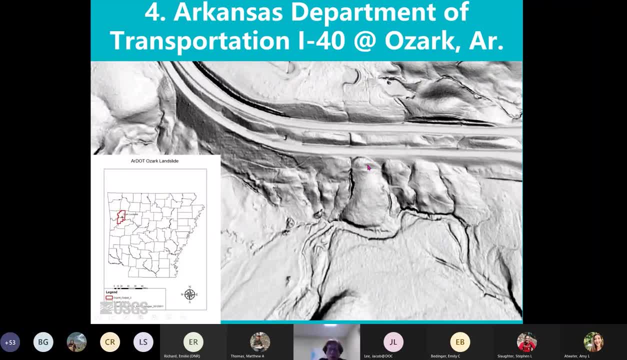 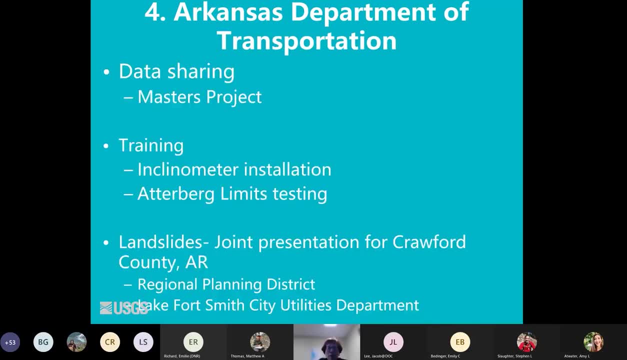 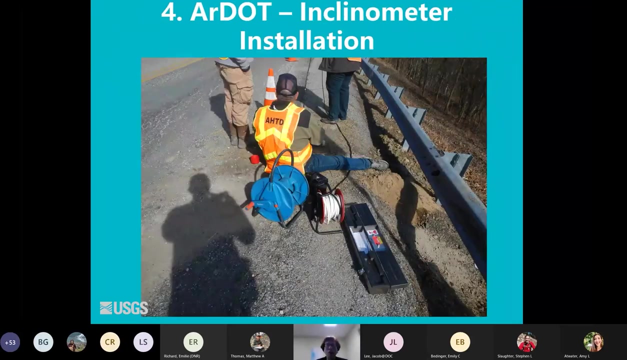 within the material loses its strength, and so what they have talked about is putting in drains there to reduce the torque pressure. some other projects are, as I mentioned, their work. we're working that highway department on the master's project and also inclinometer installation. so here we are working with them on installing an inclinometer along the highway right. 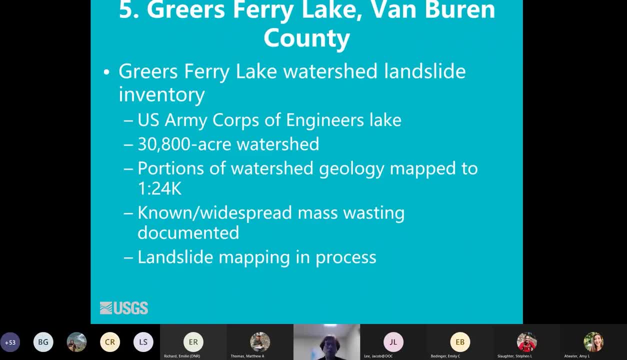 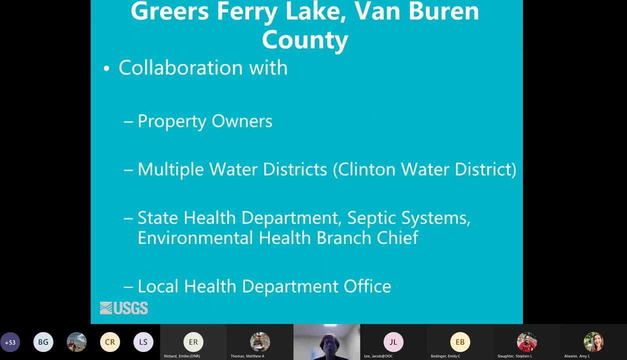 away. so this particular project, grooves free lake is is very interesting. it's I can see my really getting involved in this. so grooves free lake watershed. it's a lake, it's about a 30 000 acre lake and we've mapped part of it, part of the geology, a lot of mass wasting and we we've been working closely with property. 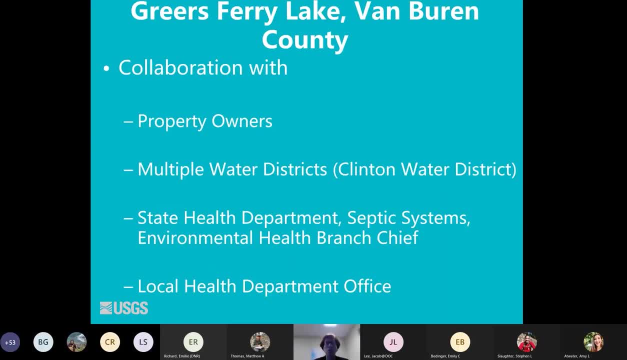 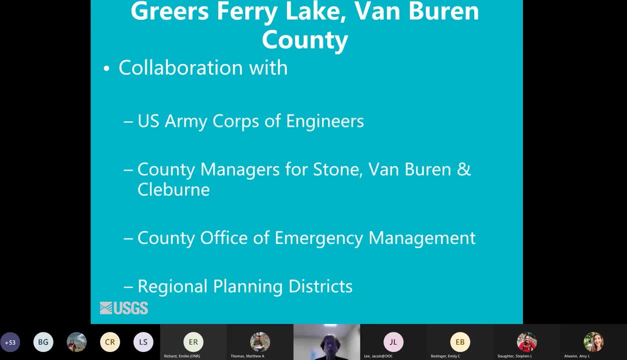 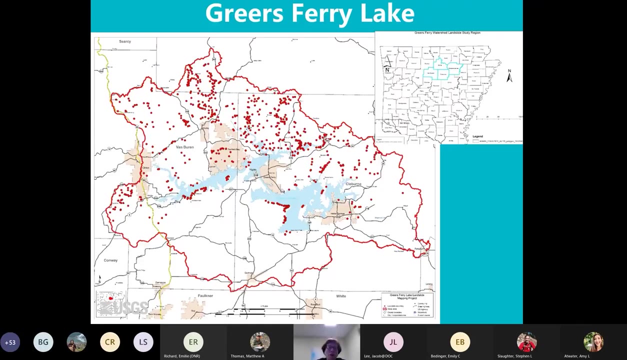 owners, water districts in the state and local health department, the sanitary sanitarians and the county managers the office of emergency management in their regional planning districts. so we're not done mapping, but all the red dots are landslides that we've identified. surprisingly maybe not, there is a fault that runs right through the lake and 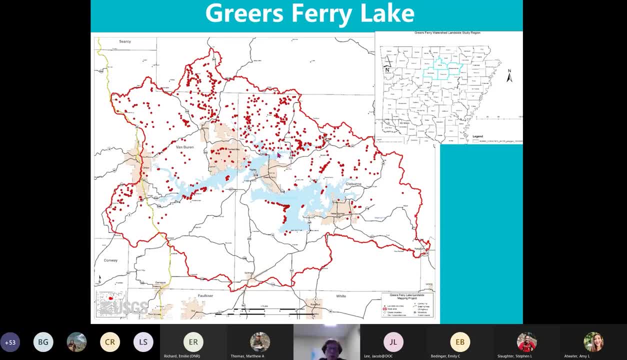 and this- I'm mentioning this because this is an area of the Fayetteville shale play, which is an area where actually, Arkansas was one of the first, first two in the nation to associate and do seismicity with well, earthquakes with deep well injection, and so this is one of the areas 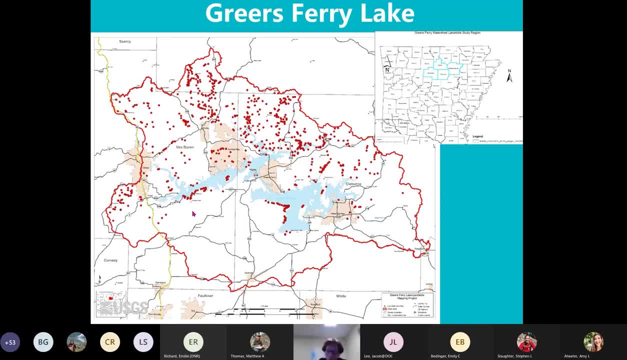 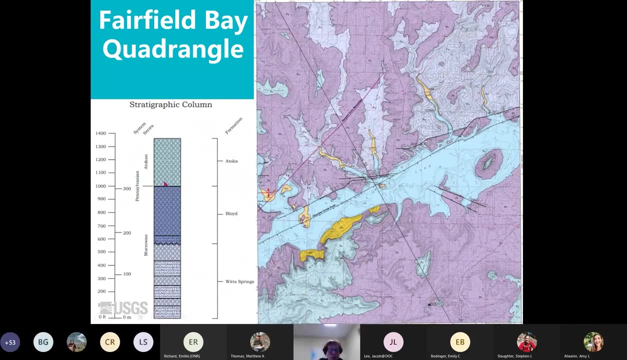 where some of the earthquakes were running in through here. so we're going to focus in on an area right down here. This is called the Fairfield Bay Quadrangle. So again, here's the geology. Again, the Atoka is present, the Bloyd is present, and both the Atoka and the Bloyd is shale as well. 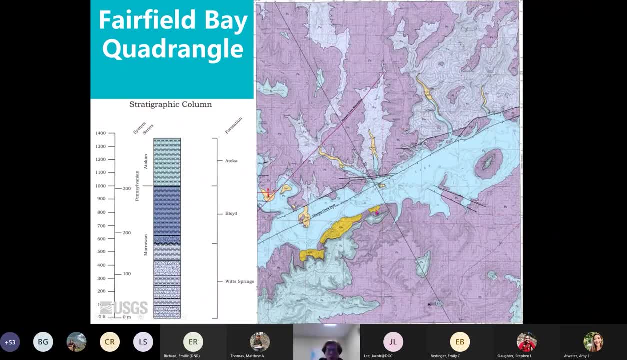 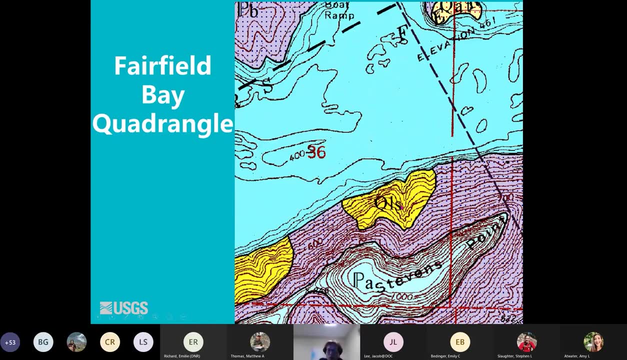 silty shale lithology, And again, we're going to move down here. This light blue is going to be the lake itself. So we're going to again focus in on this landslide right here. So the purple is the Bloyd, the light blue is the Atoka, And here is what we're talking about, going to be talking. 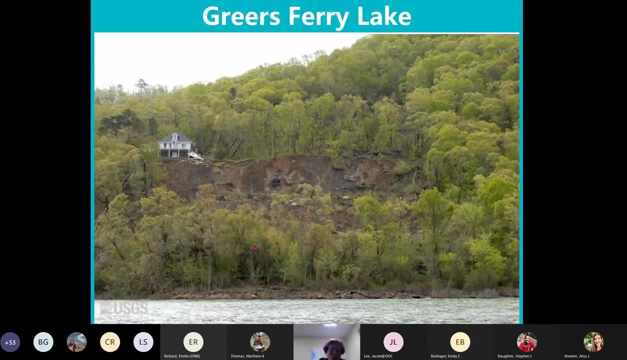 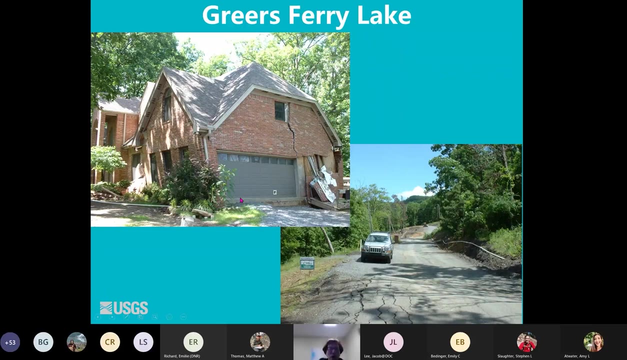 about. So this house was pretty well uninhabitable after this happened. So this occurred within the Bloyd. As you can see, the house is pretty much uninhabitable And the reason why I have this picture in the lower right hand corner is because of the fact that the house was pretty much 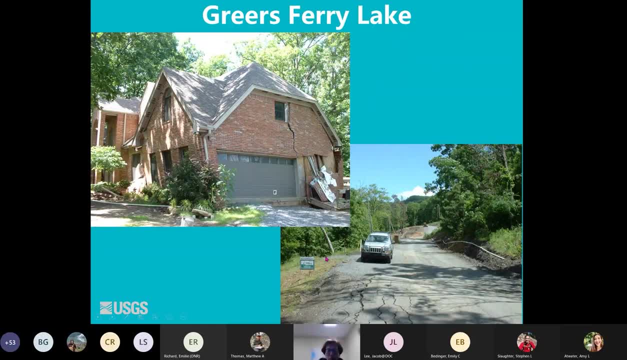 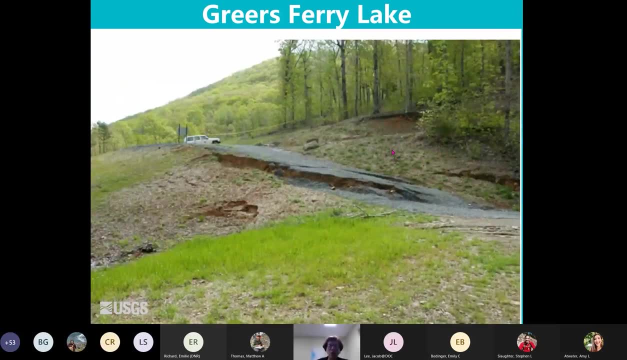 uninhabitable. And the reason why I have this picture in the lower right hand corner is because of the lower right, is because I want to point out to you this little for sale sign. So what happened with this house is the road was there, but the house, when they built the house, they decided to build. 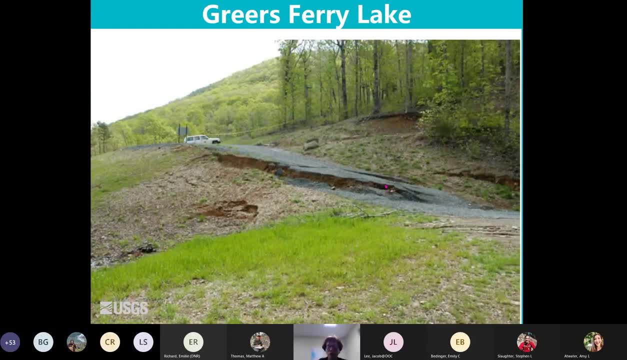 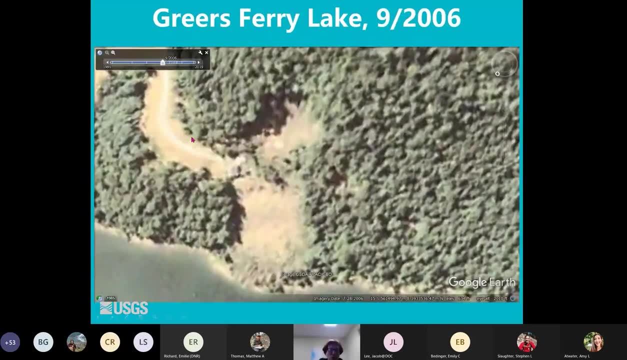 this road and put it in, wrap it around the back of the house, And I'll show you this in a minute. Let me fast forward this. So they decided to wrap this road back around the backside of the house, which caused the entire slope to fail. So here's the house here, and I'll back up a little bit. 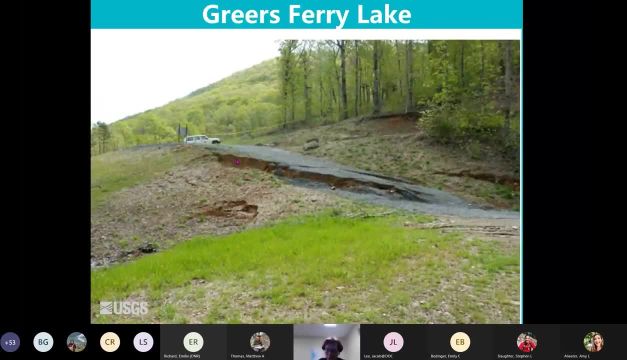 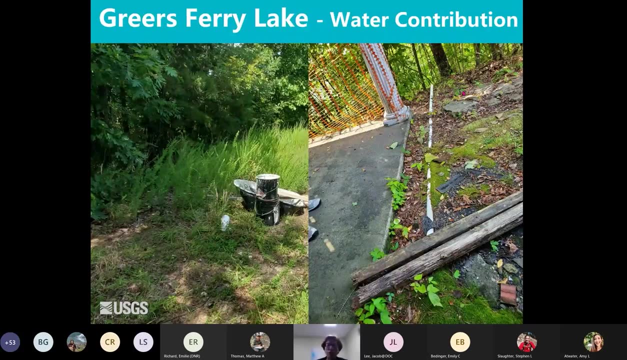 here. So that's the road coming in. And I went out there last week and, you know, wanted to look a little more depth at what's going on. So, as you can see where my pink cursor is, here and here, this is the, the scarf, the head scarf, And I got to looking around and like 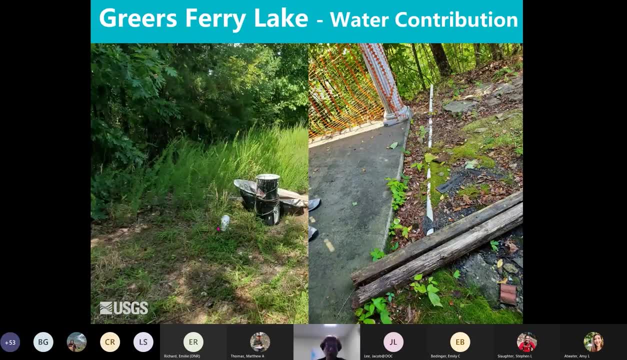 what? what is this drain line here? And I kicked this and this is a septic system. So you know that that made me think about some needs to visit with the state and local sanitarian about, about these. So here here's pictures of some of the extent of the of the. 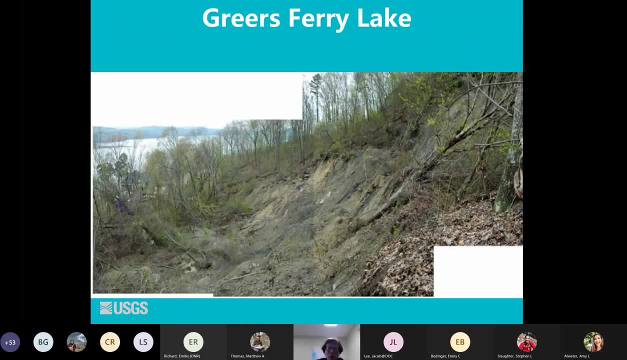 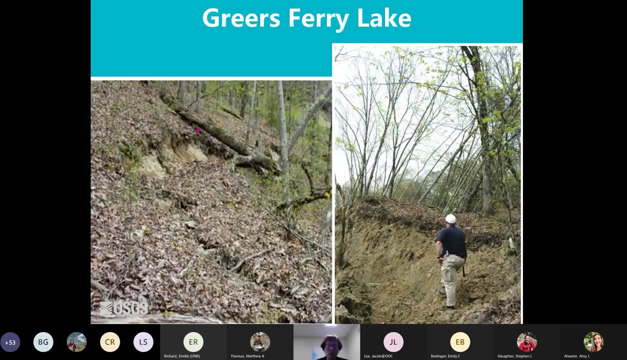 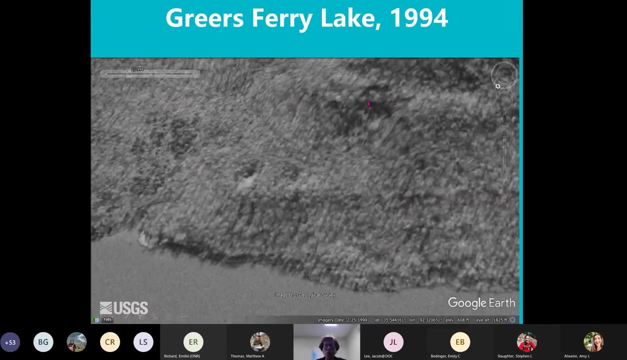 landslide Pretty pretty large, a lot of water contribution. From above you can see some translational movement here. So this is the area in 1994.. You can see it was pretty old and probably pre-existing And here's 2000.. So this road. 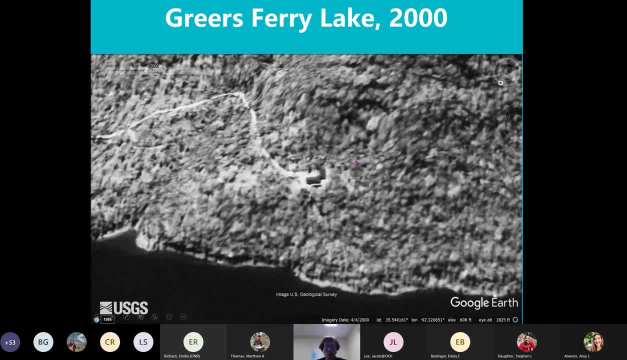 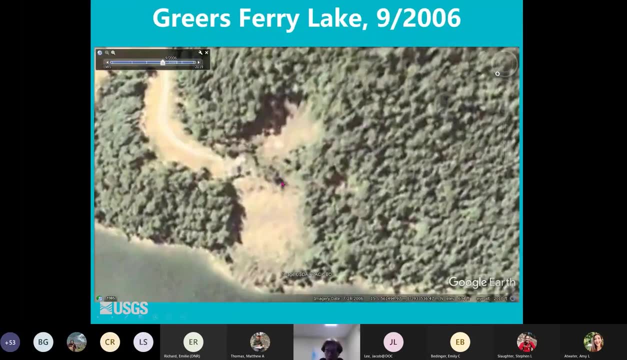 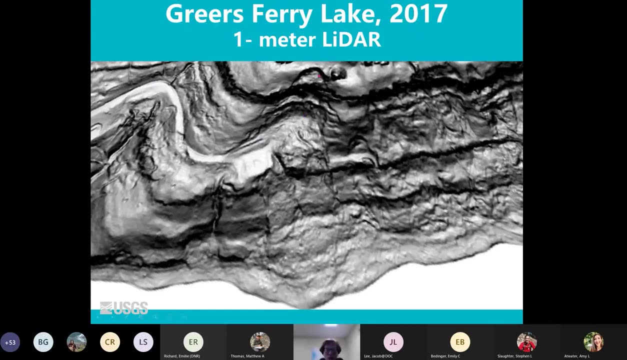 was present there and the road in the back had not been put in yet. And here it is in 2006.. It happened in March. Here is the one meter LIDAR of this landslide, So you can see it goes way up into the Etocca. 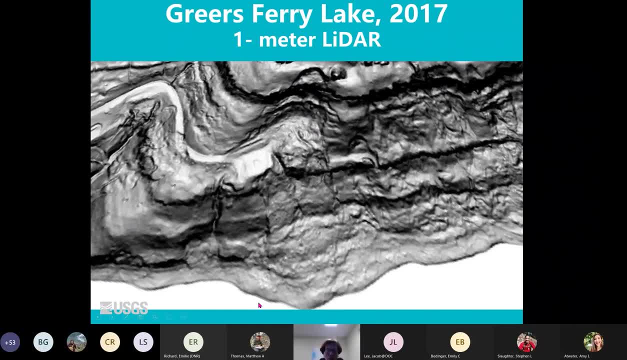 and just carries on down through the Bloyd. And so one thing I wanted to point out: it looks like they were probably a couple of things. This landslide looks like it. it comes down pretty much to the left side of the house. 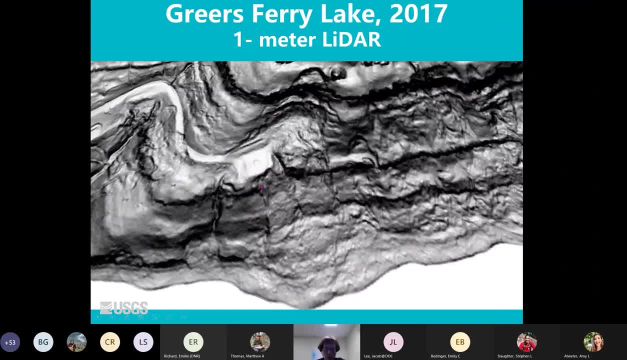 and may have had a couple of movements here. where the cursor is here, it looks like this may have been a separate movement there. so what I wanted to mention on this particular site here is we had visited with the county judge or the county administrator in like 2016. 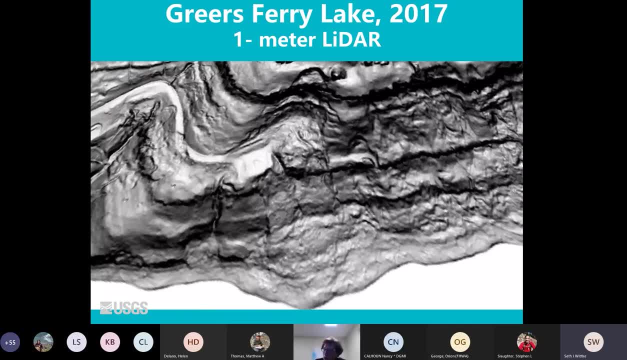 he had invited us out to look at these landslides across around the lake and he told us of a story about a family. there were five kids. parents died. kids wanted their money out of the parents had 200 acres around the lake and they were all in. 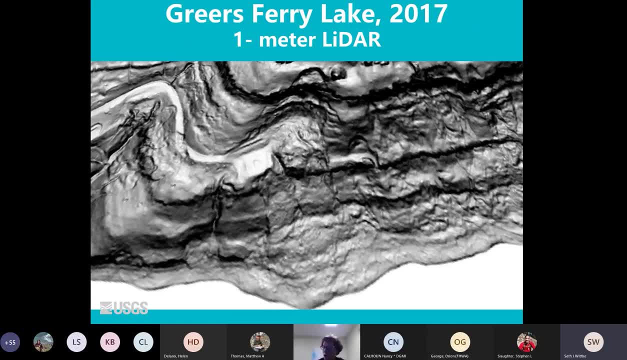 very steep lots and the kids wanted to auction off these lots in one and two acre lots and when I went out there I saw lot 36 was literally in a landslide and his hands were tied. the county judge's hands were tied because the county does not require construction permits. 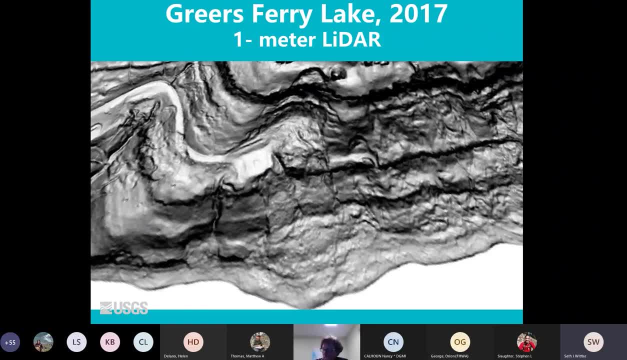 so that was quite interesting. I had a chance to visit with the local sanitarian there and they had indicated to me that typically what they do is require these homes, the septic systems, to be built on the front of the house, because people want the back of. 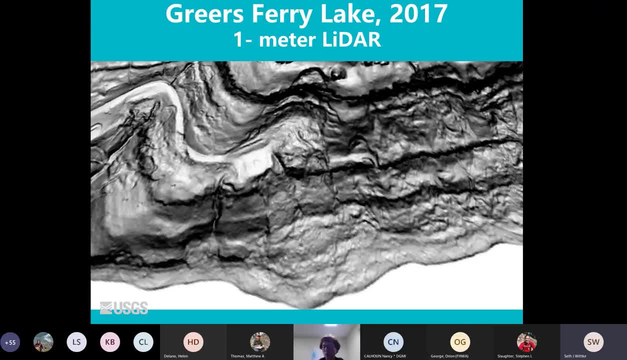 the house for their view and so. So the septic system provides additional water into the slope, So I think that's something that we need to have future conversation with the health department and the way they encourage and locate their septic systems. I'm going to be setting up a public meeting with the county elected officials. 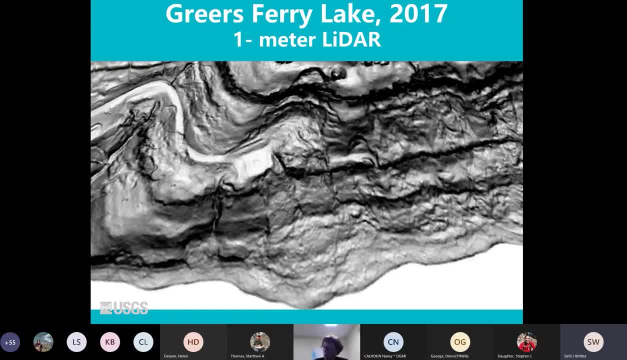 the county office of emergency management and the planning districts for an overall to educate people on the spatial distribution of these slides. I did have an occasion to visit with the people who own this house here. They want to move back into this house. The local water department will not connect their water. 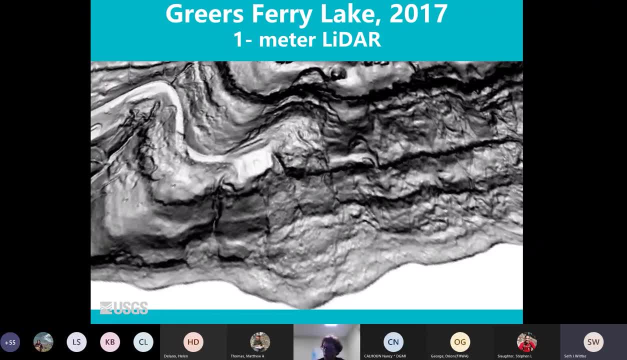 So in order to be able to live in the house, of course they've got to have water, And I'm not sure where they're going to put their septic system. So in addition to that, I also talked to the individual who bought this property just to the left side of this house. 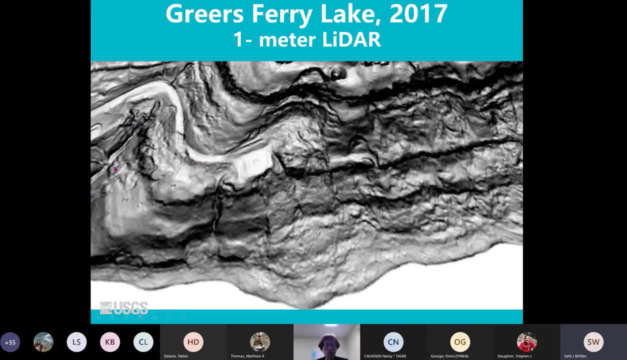 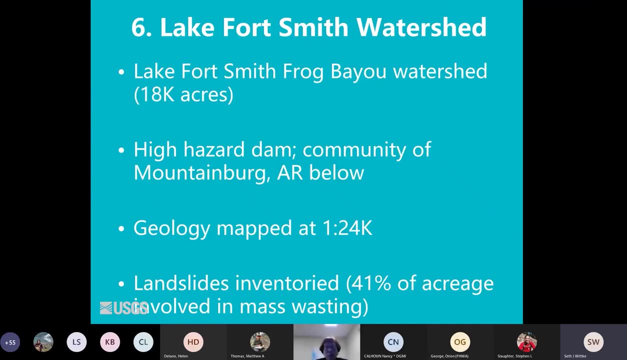 And this person was from out of state- bought this property sight unseen, not knowing it had landslides And now I believe there's going to be a lawsuit. So I'm going to talk about Lakeport-Smith Watershed. So we became familiar with this landslide from the Arkansas Division of Emergency Management. 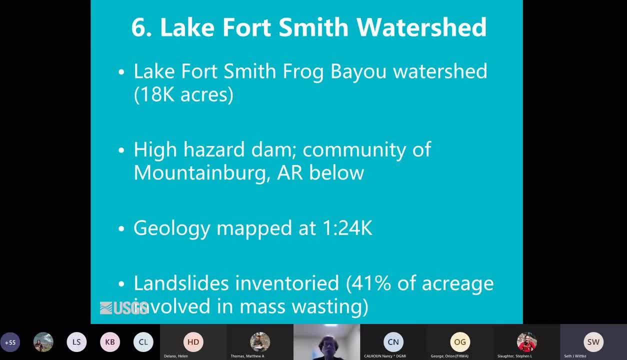 In December 2015,. there was a large rain event and a landslide occurred just below this high hazard dam, And so we went out. We went out there to look at it. What we found was that, after we inventoried everything, there was about 41% of the acreage was involved in mass wasting. 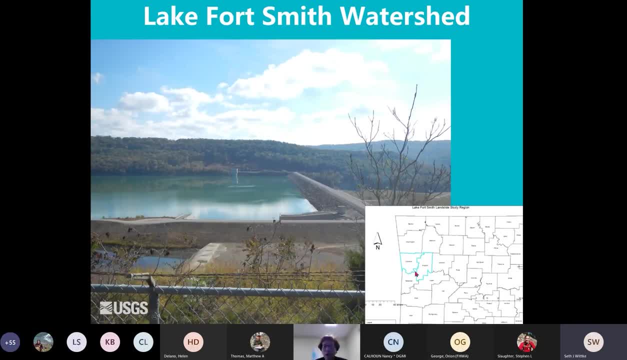 Here's the dam. This watershed is in the western part of the state, near Fort Smith, So we're looking at the dam and we're looking to the east. So there's the water intake down here. on the bottom is the emergency spillway. 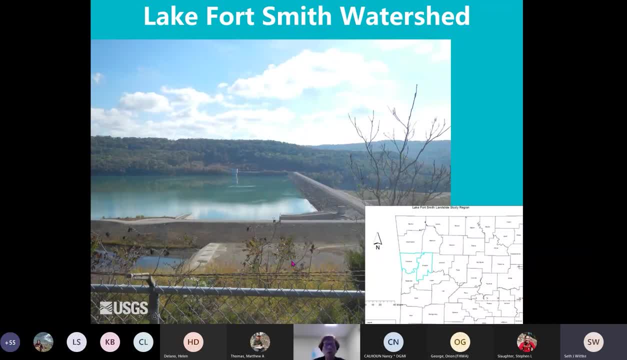 They had. this is a water supply reservoir which was built by the Fort Smith City of Fort Smith Utilities. They revised and updated the reservoir to raise the elevation of the reservoir, So the dam put in a new emergency spillway and that construction has caused some some issues. 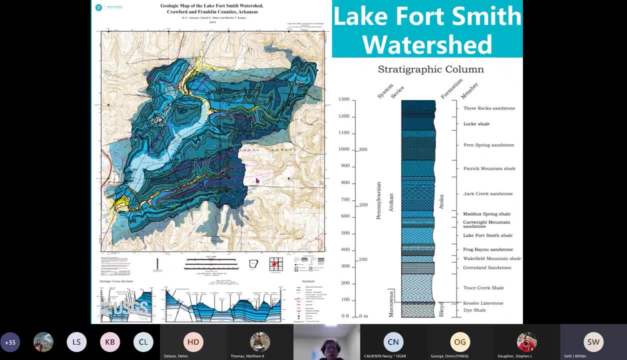 So what we did was my staff went out and did a geomapping project and also map the landslides, And we did this a little differently because the Atoka is an undifferentiated formation. We considered Describing the strata lithologically because it's undifferentiated. we wanted to see about correlation elsewhere and, as you can see again, this is all Atoka here and at the bottom here you can see highly structurally influence. a lot of faulting in here. 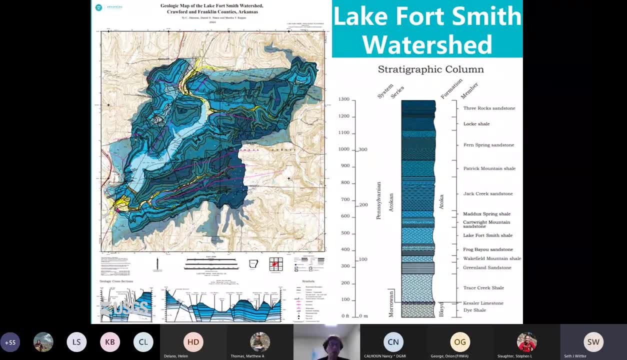 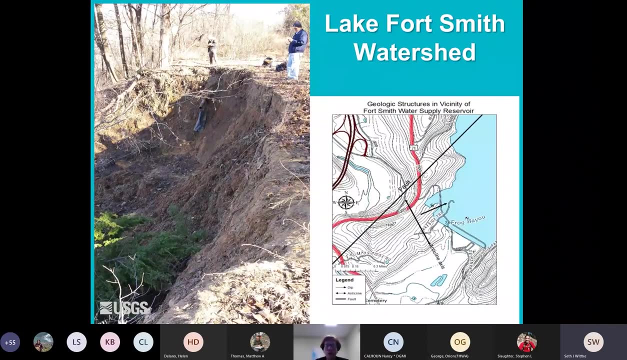 So imagine, if you will, a high hazard dam with a lot of faults going through. Here. there's one fault which is regional- It's called the Drake Creek fault- which runs kind of northeast and southwest. So here's the landslide that we were called out for in December. 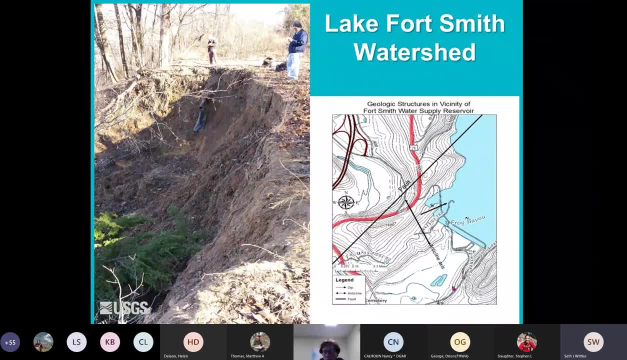 That landslide. I'm going to show with my cursor down here in the lower right hand corner, which is where the landslide occurred. This is the emergency spillway up here and, as you can maybe see, there's this highway, this red here is Highway 71, and the emergency spillway was put in right through here. 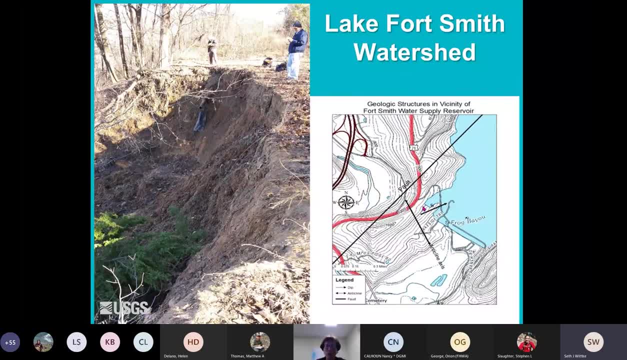 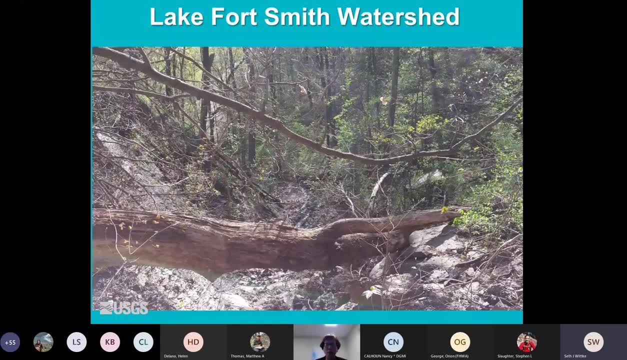 And so what's happened? I'll show you that in a few pictures here. So here's some landslides in the watershed, pretty high up in the watershed, pretty steep, a lot of creep here. So here's some landslides in the watershed, pretty high up in the watershed- pretty steep, a lot of creep here. 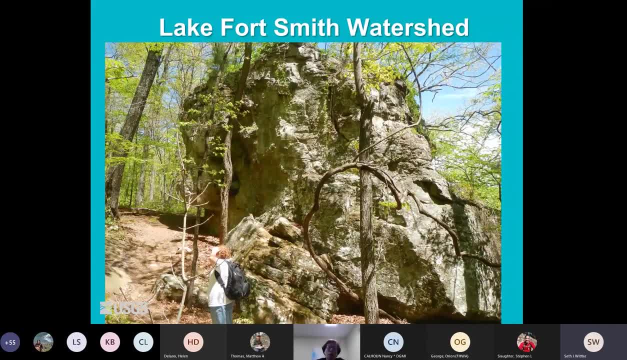 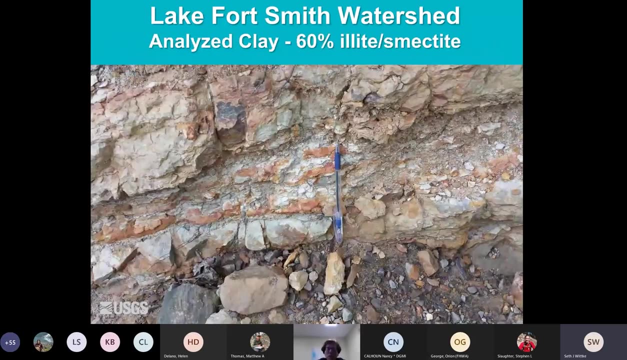 This is a boulder which has come down from one of the hills. Here I am for scale. This is part of one of the Atoka sandstone layers that's fallen down, And this particular layer here is a clay, And it's found in three different areas within the watershed. 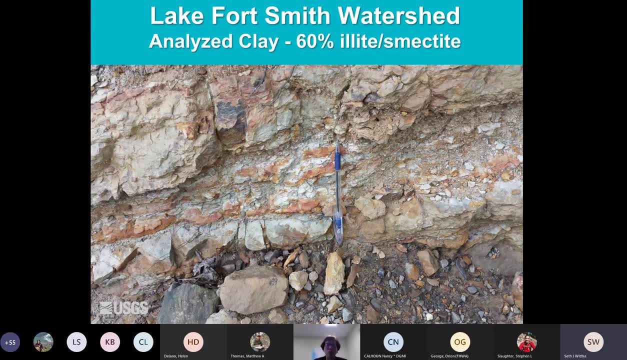 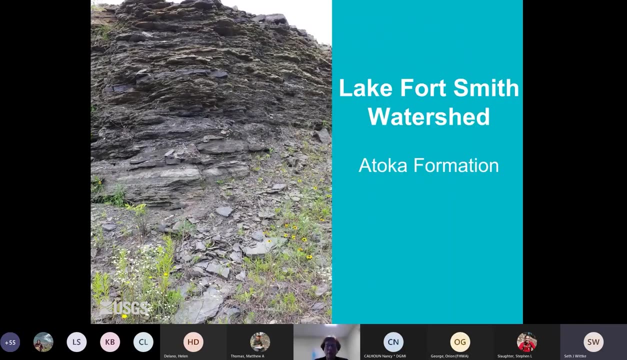 in all three different depositional environments. We're hoping to maybe use that for correlation, but we're not able to. And we had this analyzed and it's 60 percent illite smectite which could definitely contribute to some of the movement. 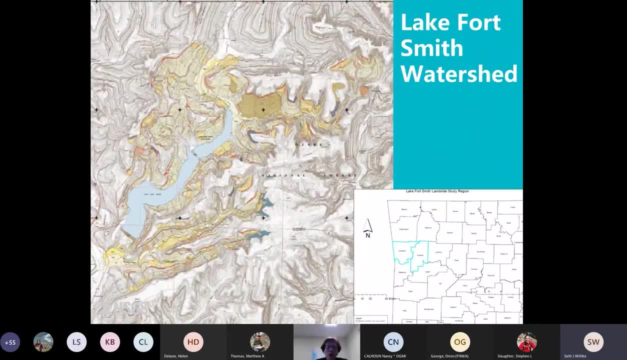 This is what the Atoka formation looks like and this is a map of the Lake Fort Smith watershed And I'm gonna kind of- I apologize, I apologize, the boundary, the watershed boundary, doesn't show up here very well, but my cursor is kind of going around the 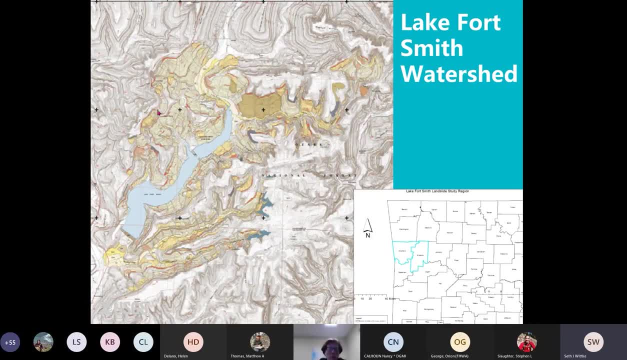 outside of it Watershed. So we identified the landslides here, have identified them based on the age and the type. So the red here is a headscarp And these different yellow colors are the different types of landslides and the ages as well. So here is. 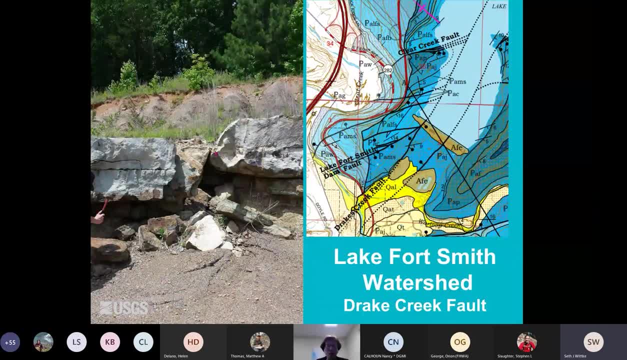 a close up of some of this faulting, And this is a. there were a lot of grobbins in through here. This is a really nice example of some of the faulting here. Here's the Driggs Creek fault that I talked about. Here's the dam here And here is. 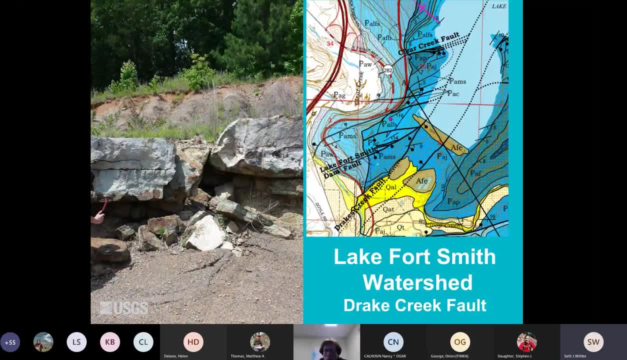 71, this red line here. So what what has happened is, when they elevated the dam, they had to cut a new emergency spillway, And so what that did was cause this TOCA to start failing, And you can see it failed for. 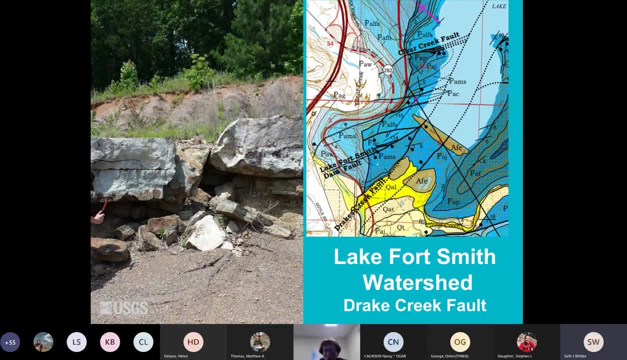 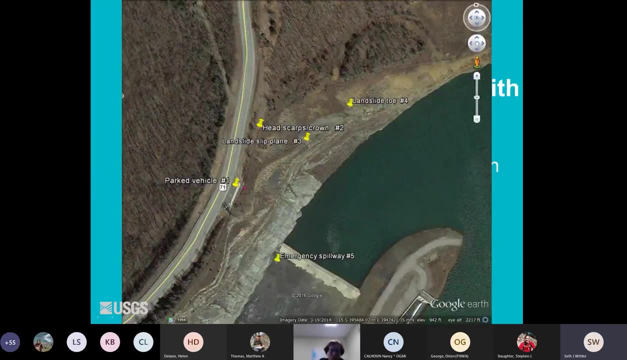 several reasons. There's some faulting here. After they had to cut this they became the engineering firm became painly aware of how much faulting there actually was in here. So here's a better picture here. So here's the new emergency spillway they had to. 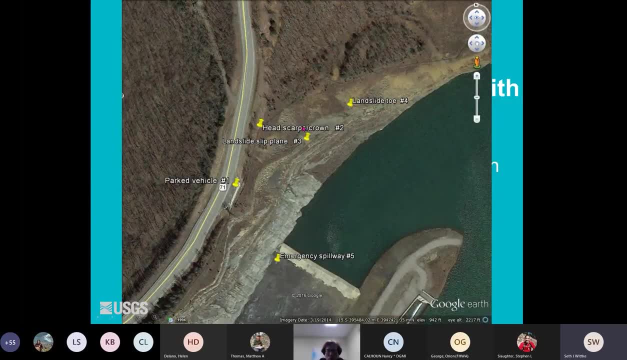 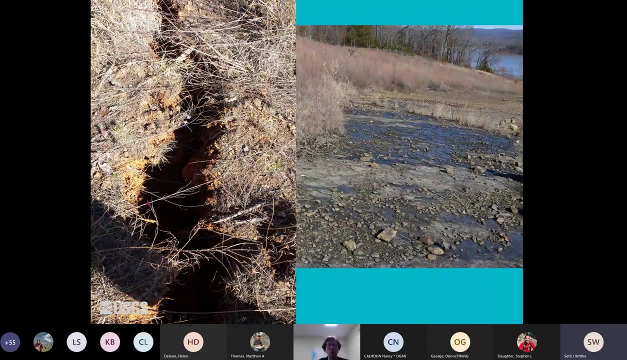 cut all this out. So we identified some headscarps, And what's happening is now these headscarps are encroaching onto the highway- highway right of way, So that's a concern. So here's these scarps. I was telling you about headscarps. 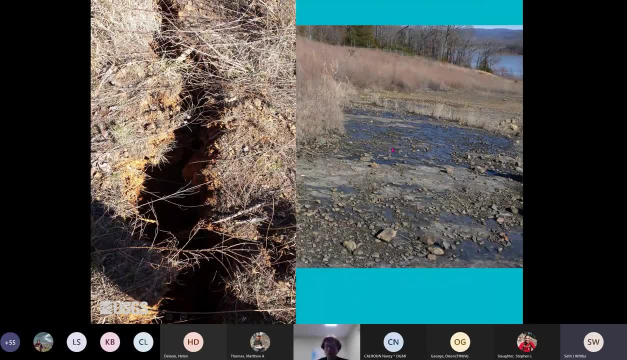 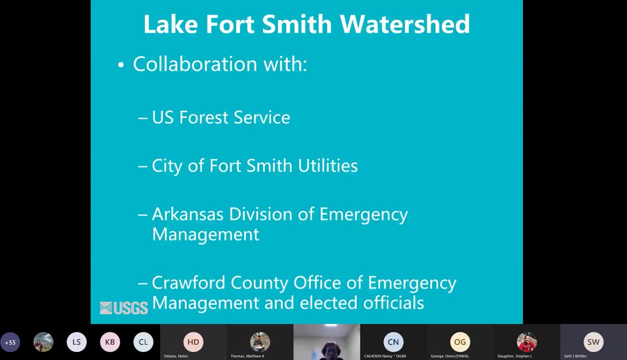 right near the highway And here it is draining some of the water. As I mentioned, we're working with the Forest Service majority- I'd say 60% of the properties around the lake, our US Forest Service- And we're also working with 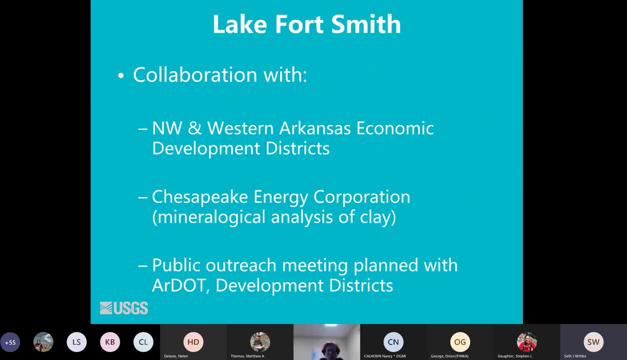 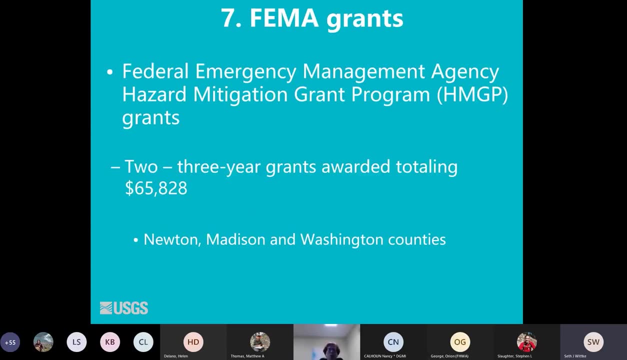 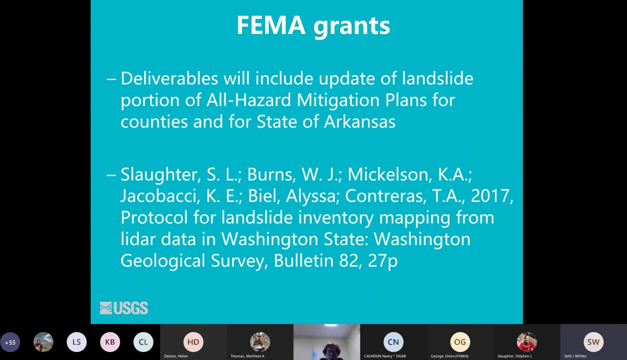 planning and development districts in in these landslide inventory. And another project we're working on are these FEMA grants that I talked about. we have two three year grants totaling about 65,000.. It's covering Newton, Madison, Washington counties, which is in the northwest part of the state, And our 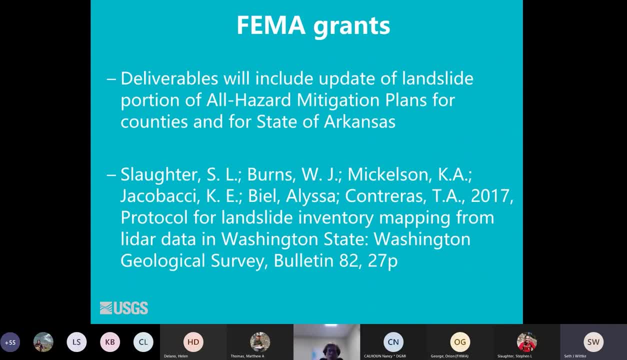 deliverables are going to include an update of the landslide portion of the all hazard mitigation plans for the counties and for the state And we're following the state of Washington Bulletin 82, and our protocols for mapping these, doing the landslide inventory. So these are. 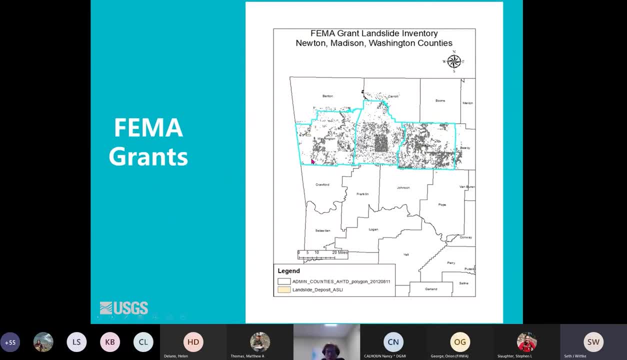 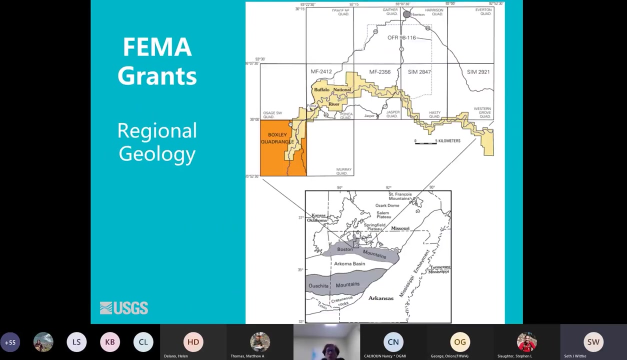 the three counties that we're mapping The shaded gray. this was prepared some time ago, So the shaded gray areas are areas that have been identified as mass wasting. We're not done So, so I wanted to show you the geology of this. 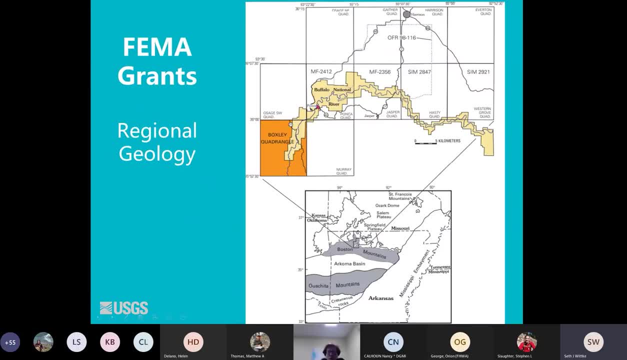 area. If anyone has ever floated on the Buffalo River, We've been able to do landslide inventory in several quads along the Buffalo. it's a beautiful stream to to float in there. So this is in the northwest part of the state And we're going to focus. 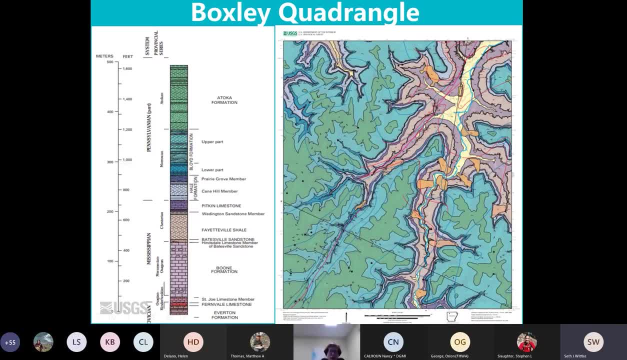 on Boxley And we're going to focus on this area here And we're going to look at the, the the. these strata are relatively flat line And, as you can see, the majority of the area is covered in these susceptible strata. The USGS mapped this and they identified, So these. 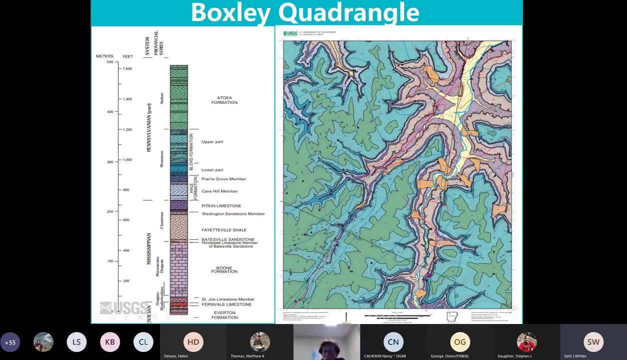 orange blobs, polygons. in here are the landslides that the USGS mapped And we are in going through these quadrant groups. we've been able to extend many of these footprints of these landslides And, and I can say I haven't actually done- put a 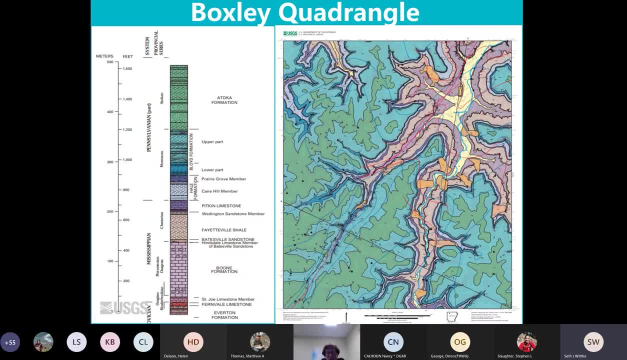 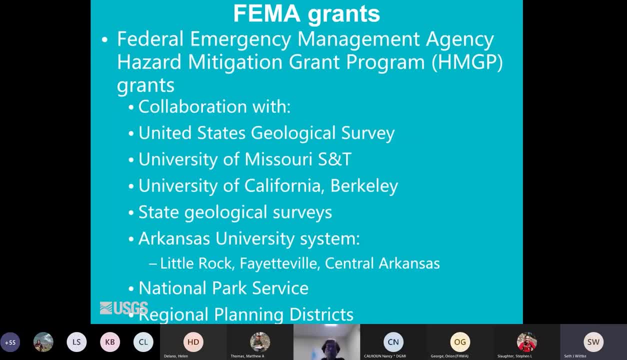 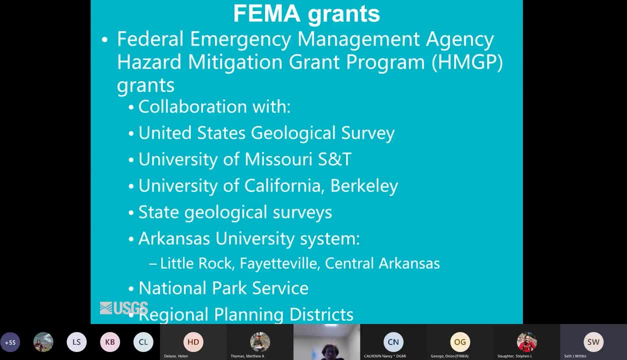 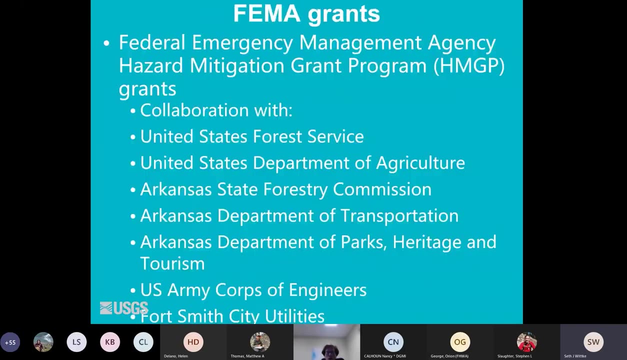 been extremely helpful. Like I said, University of Missouri, Science and Technology, California, Berkeley, other states, Geological Survey, National Park Service, Planning Districts, Forest Service, and on that We've also worked real closely with the Fort Smith City Utilities. We're going to share our ship files with 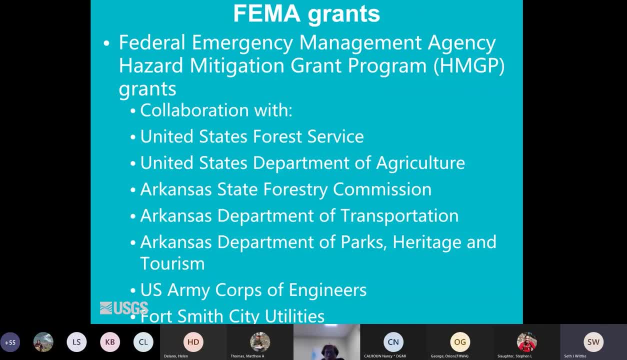 them and uh helping them out with, because, uh, when that event happened in 2015, um, their watershed, or their lake, of course, it's a water supply reservoir and it has to meet ep drinking water standards, so, um, they were not able to meet the opacity and, um, uh uh standards, so it took them. 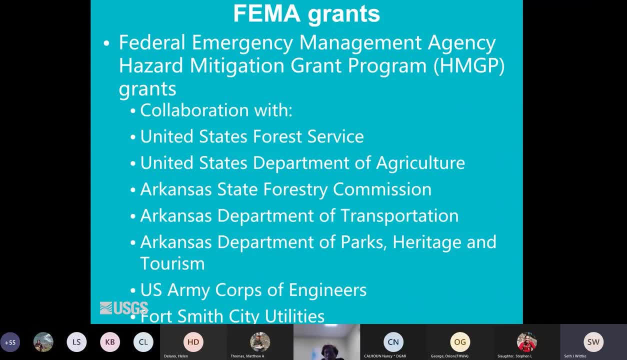 two years to get back to um meeting the um, epa drinking water standards, and so, um, this is going to help them manage their watershed. they, they own all the land immediately around uh, the lake. um, but of course, you can't manage things uh uphill. um, and what i wanted to do here, 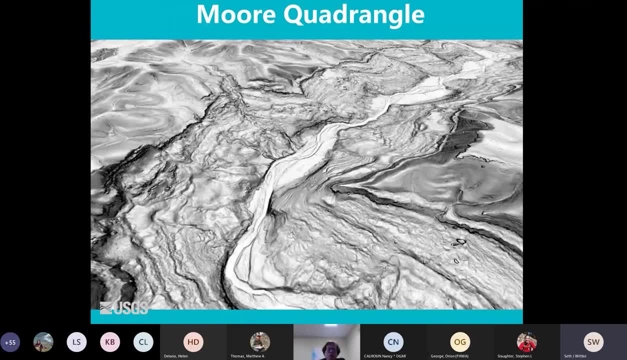 these next three slides are um taken from globe, our globe, at an angle, and so i just wanted to point out to you the spatial distribution of the mass wasting. this is in the moore quad, which should be just uh, east of the boxley quad and uh as as one can see. 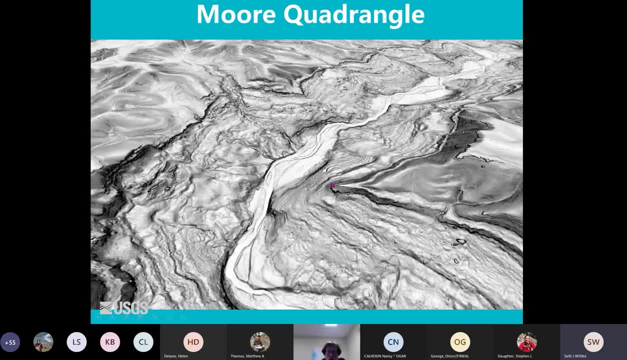 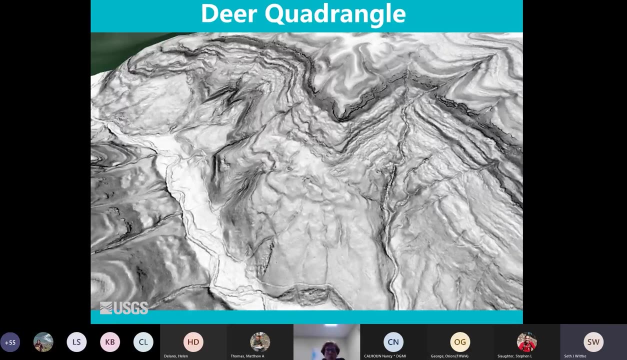 entire slopes are, uh, uh, have been affected, uh, by the, the um mass wasting. so this is the moore quad. um, here's the deer quad, which would be a little bit south and east um again. um, here's some slides here. um, here's some here. and then this is the boxley. 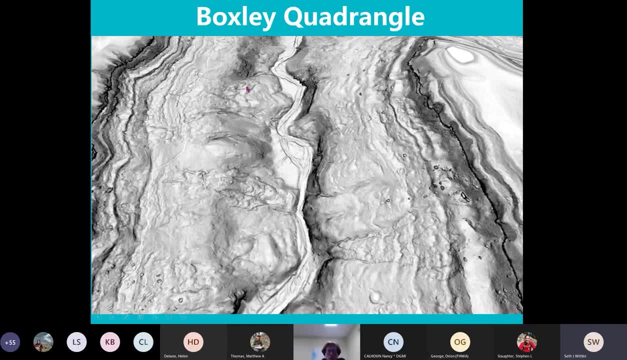 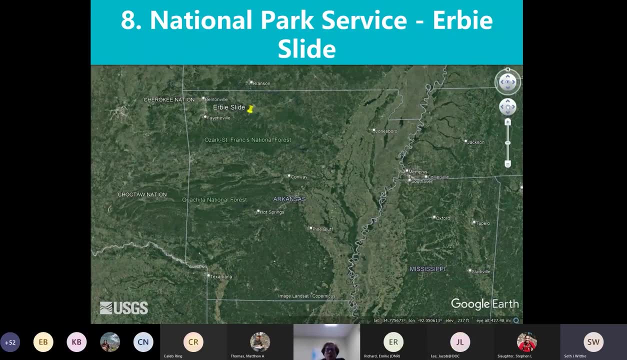 um a little bit different orientation where we could see a lot of flow in through here, and so the um national park service, as i mentioned, is another um organization that that have been very helpful. we went out to visit the irby slide back in april with them and also with the university of arkansas. 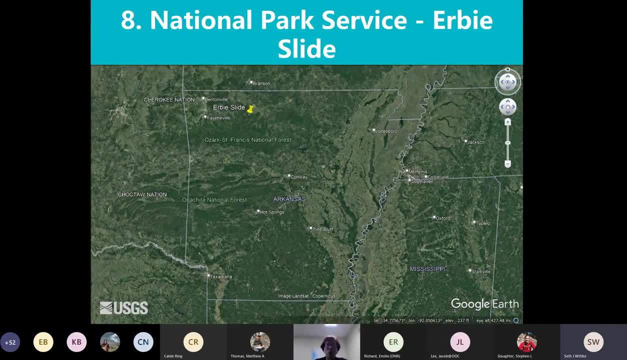 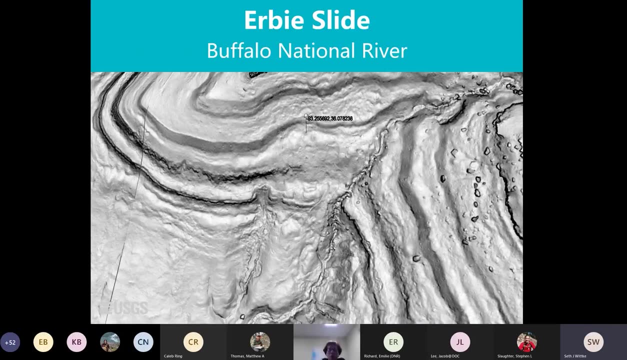 at fayetteville, one of their professors and graduate students. we're probably going to be going out there next, uh, next week, and this is a reactivated slide. you can see this was an old large slide and, um, we went back. like i said, in april. identified the slide uh headscarf as being up here. 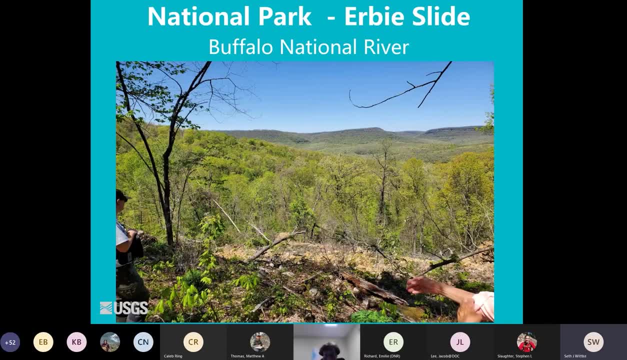 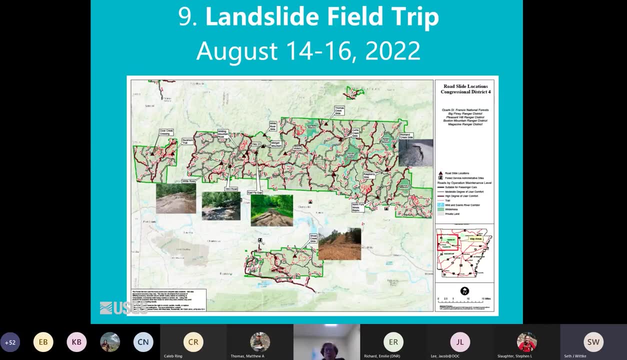 this is the slide. this would be looking to the northwest um, and so our our last um thing i'd like to mention is um. next sunday we're going to be- or this coming sunday we're going to be- having a field trip with one of the professors from university of missouri science and technology and his phd student. 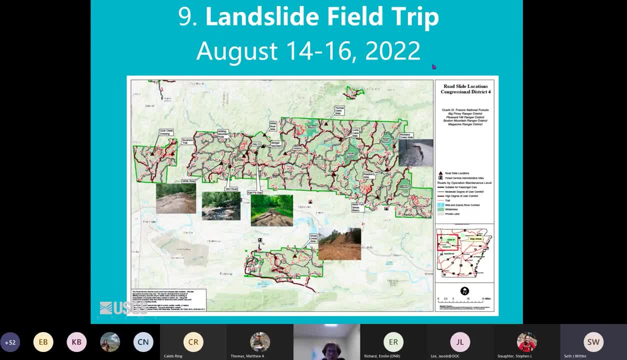 when we're going to visit about six slides in in arkansas, and the reason why one of the reasons are coming down is, um the phd student had his dissertation, has his dissertation in nine quads uh, within newton county uh, which is boxley, which i just showed you. um, this particular map is a us forest service map that 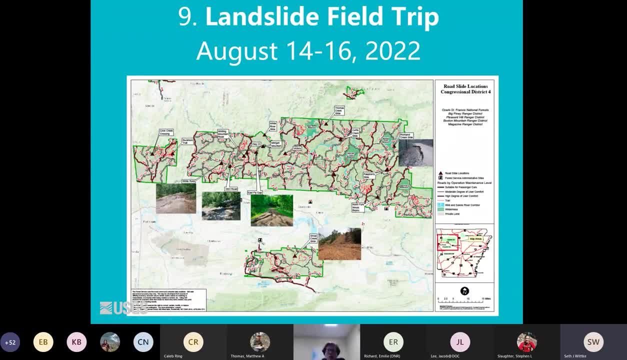 was presented to the us congress last week by us forest service um just giving the congress an update on the slides um occurring um in arkansas on on the us forest service, and so we're going to be visiting um, so my contact within the us forest service is going to be. 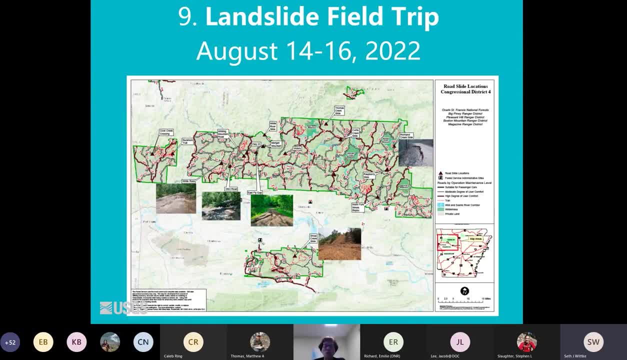 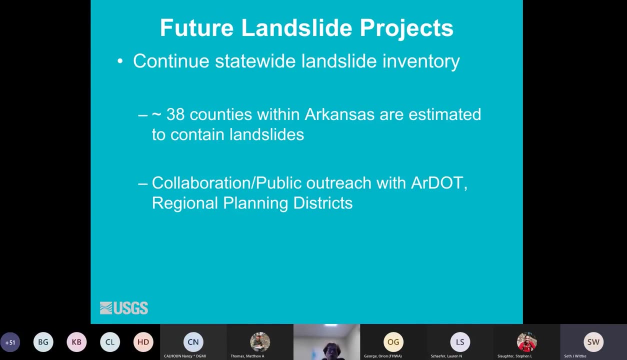 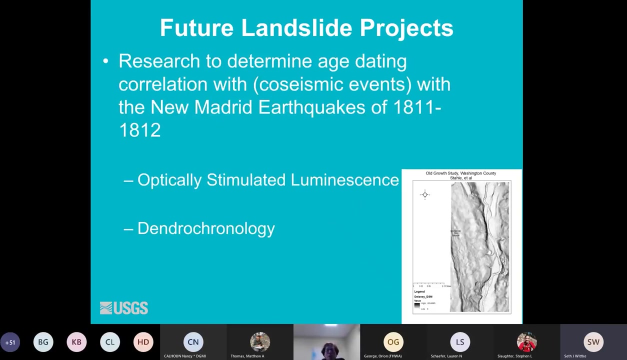 um coming meeting us at um several of these slides, and we're going to be visiting those, as well as the one in the national park service, and so some future landslide projects that i would like to uh work on. um is uh, what what i'd like to do is to see to age date some of these earthquakes, to see if there is. 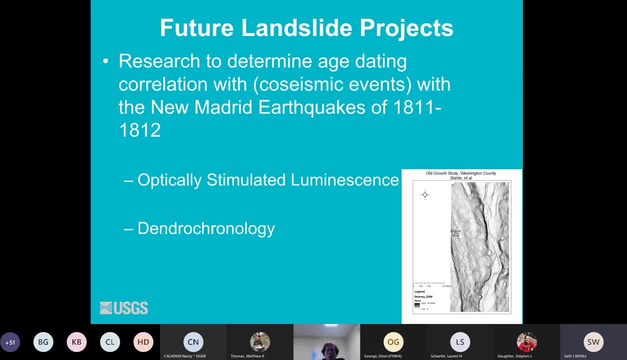 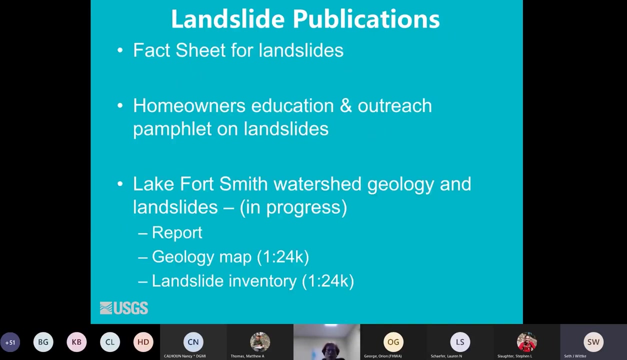 um a common age with, uh, the pneumatic seismic zone. um, we're looking at possibly doing an osl testing or dendrochronology. i've reached out to three professors whose specialty is dendrochronology and they're they seem pretty excited about it. so, um, we've done some publications. 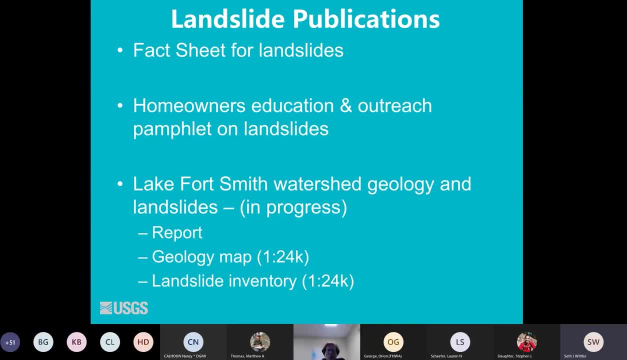 um some fact sheets for landslides for homeowners. we've got the um the mapping at lake port smith, the map for the geology and landslides. that's in progress. we're going to be doing a report and including the maps and all and we're also we 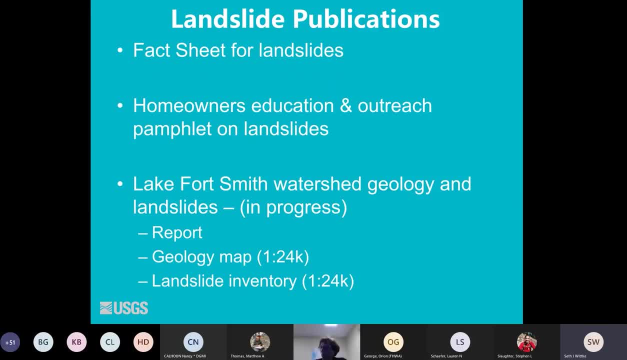 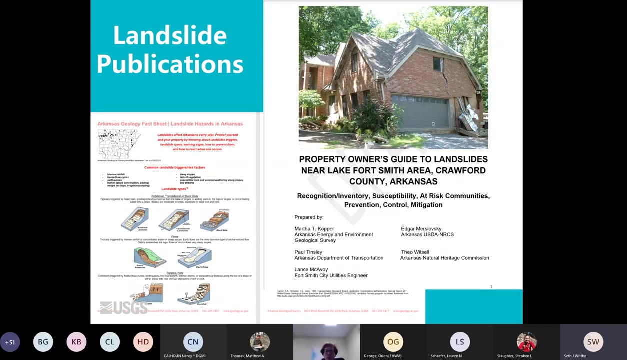 had planned to do a uh, an outreach with a highway department, um, and then pen, the pandemic came along. so that's, that was kind of put on the back burner, but we, we do want to do that again. this is our one of our publications: um, on landslides. 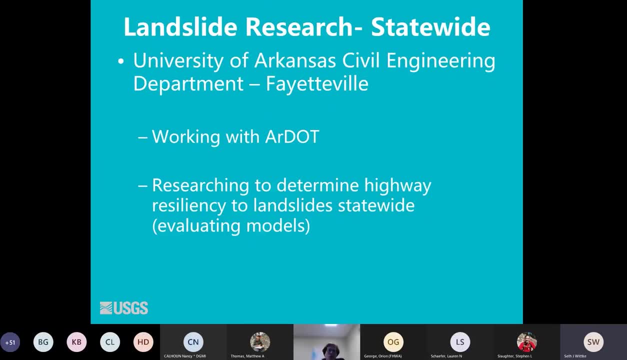 um. so some other landslide reach research going on in the state? um i know university of arkansas at fayetteville um they're doing some research on uh highway resiliency- how resilient the the state highways are to landslides and liquefaction. um also the geology department. 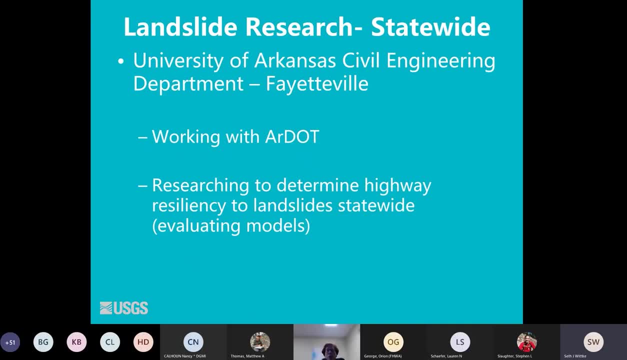 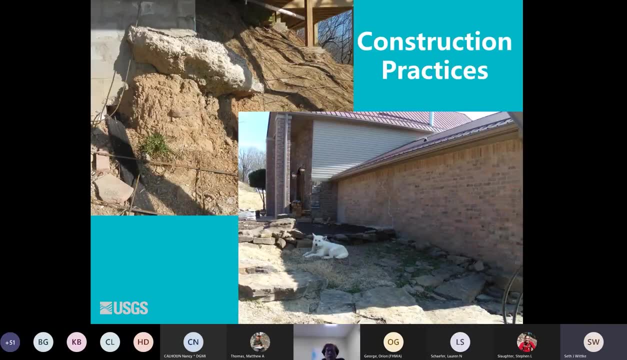 is doing uh some research on the movement of the the boulders, how they the boulders are moving downhill and um, just as a point of uh information, this is uh lake sequoia, southeast of fayetteville, and it's kind of interesting how they design and build their houses. 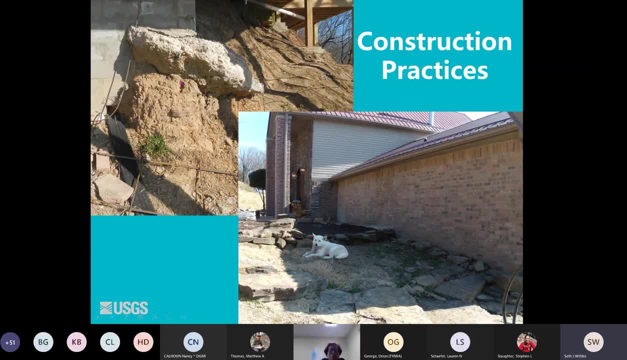 where these people complain about a landslide on their property. this is an in-place boulder and they just put their cinder blocks right on top of that boulder and when we got there, they were doing construction- uh, repairing some cracks. this is an addition, this is the original. 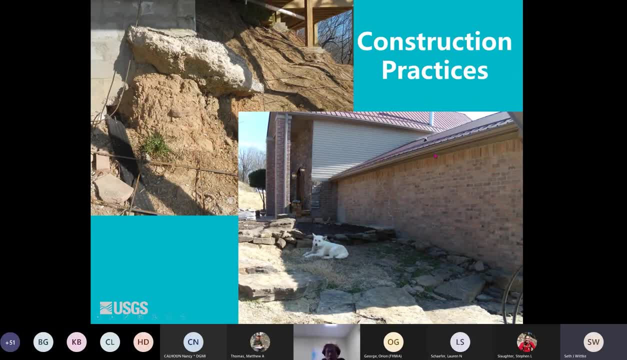 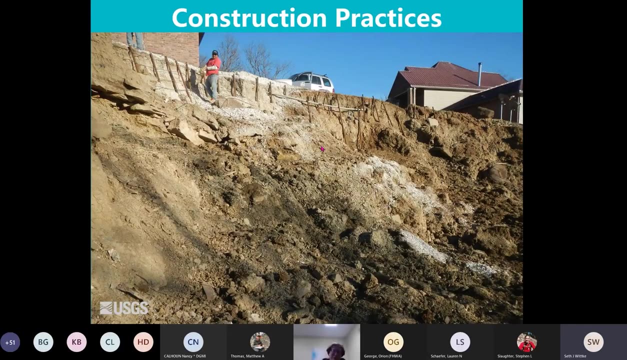 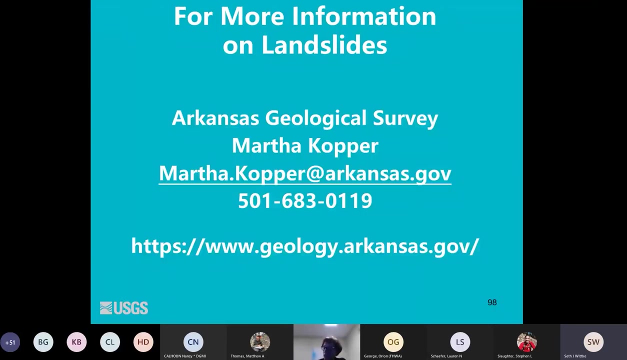 house. this is the addition. they were doing cosmetic repairs to this addition and i got to look in it, look at that crack and look at this construction, and then here's how they're repairing the landslide. so kind of funny. so, um, what i'd like to do is just to thank all those who have helped. 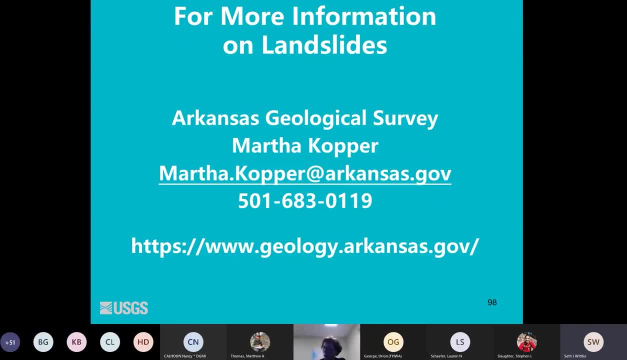 helped in the development of of our program, um, usgs, oregon geological survey. uh, really appreciate their, their input, contributions and um- and i do welcome some- any kind of input suggestions on on any of our programs. so thank you.